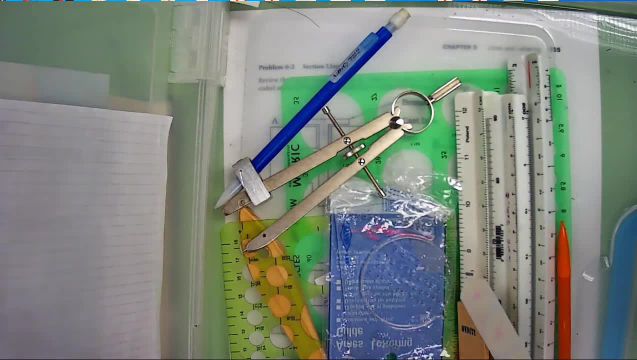 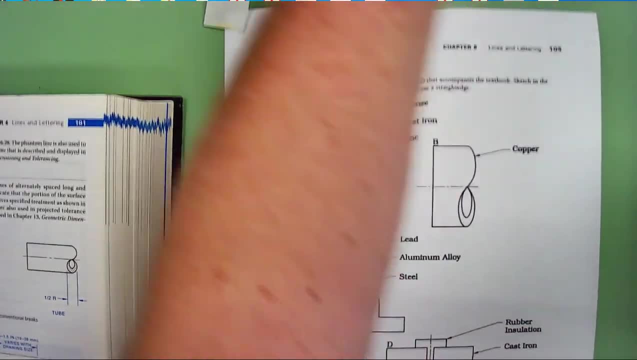 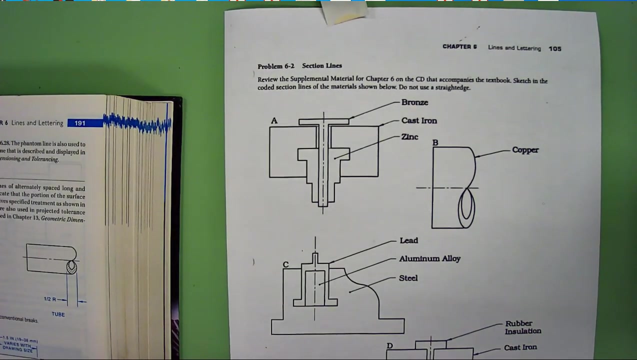 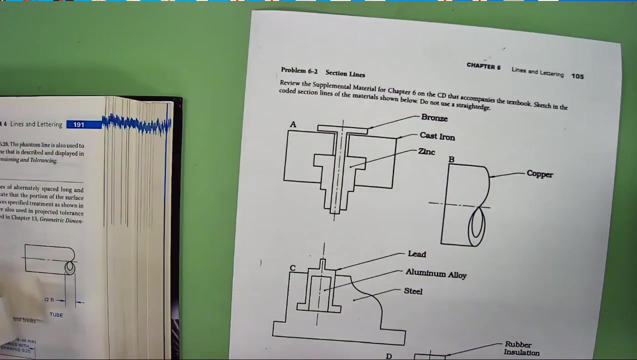 the 0.5, and I'm going to set this back up here. Actually, I'm going to set that over so it's not in the way, And then I'm going to tack my paper down so I don't accidentally move it. Let me try to get it square with the screen, because it's not square on my. 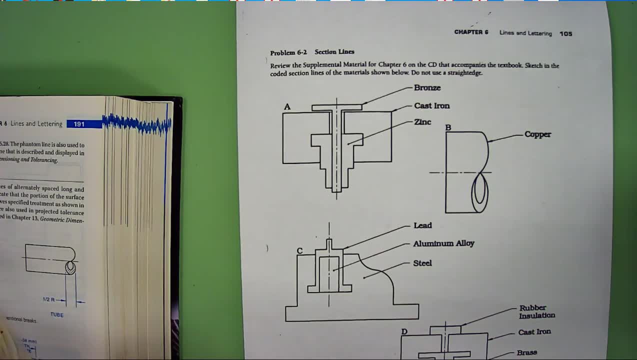 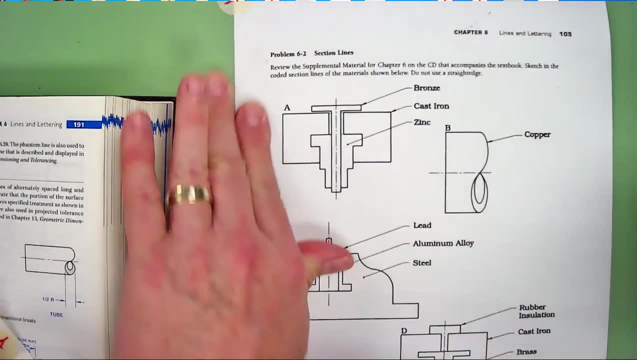 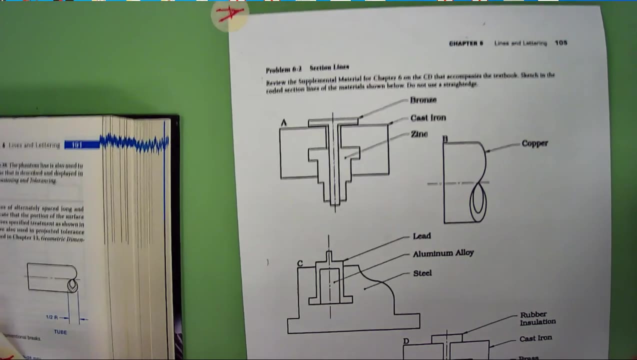 desk. That's okay. So this is how your paper should be. This is how your paper should be taped down, which you can't see either one of them. I'm going to move this for just a second. See, I've got the corner done up there, and then. 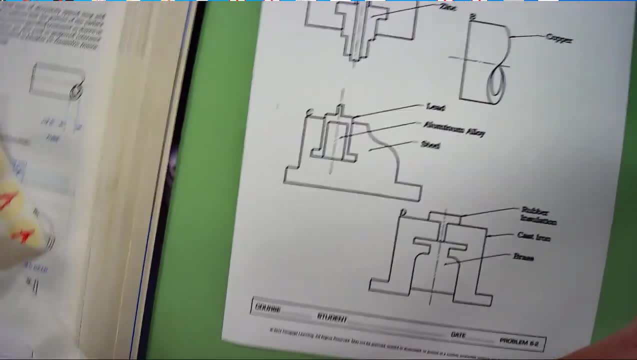 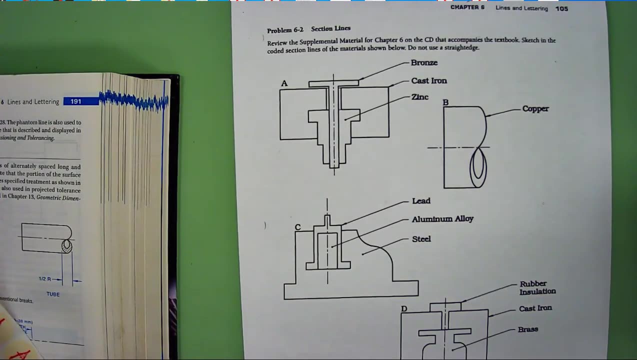 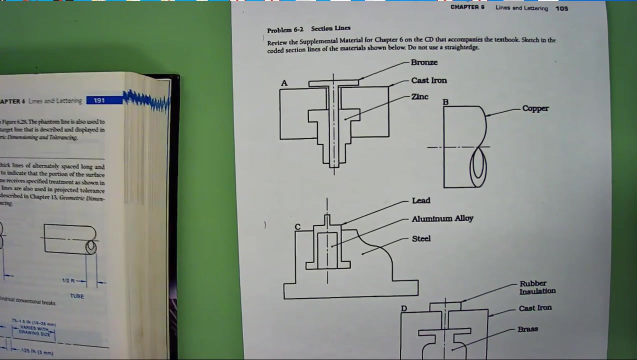 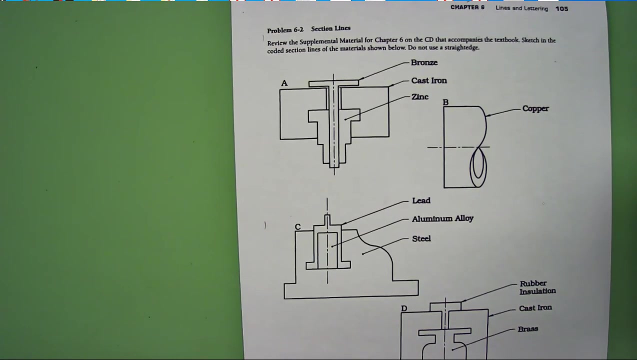 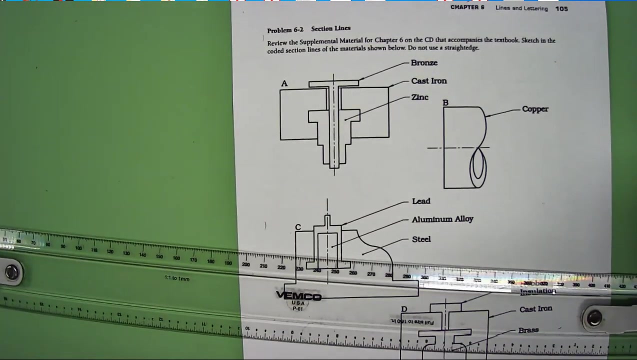 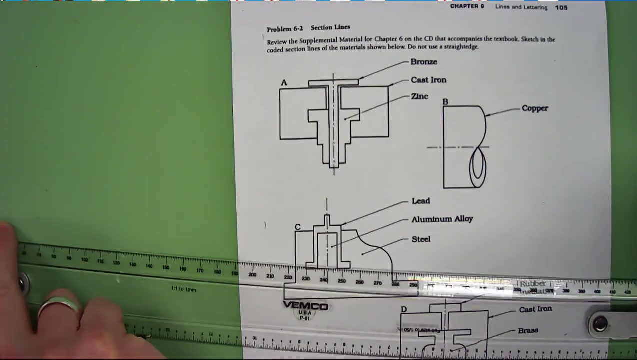 way down. yonder is the other one. The plan is to have it at all corners, but since this is just a demonstration, I'm going to show you. I'm going to put the book over here. Some of you probably have T-squares. This right here is a drafting machine, So I'm going to level it up with the paper. 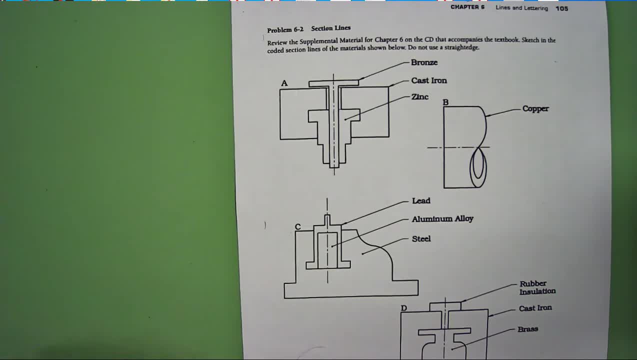 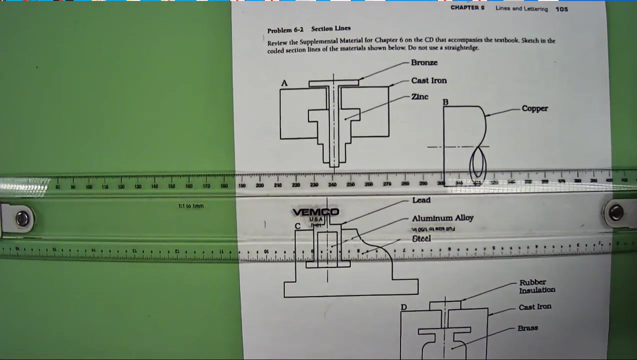 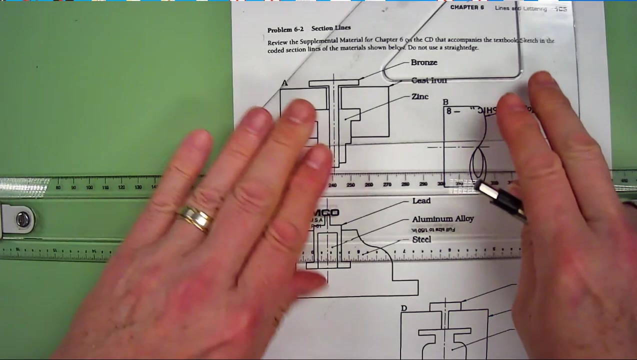 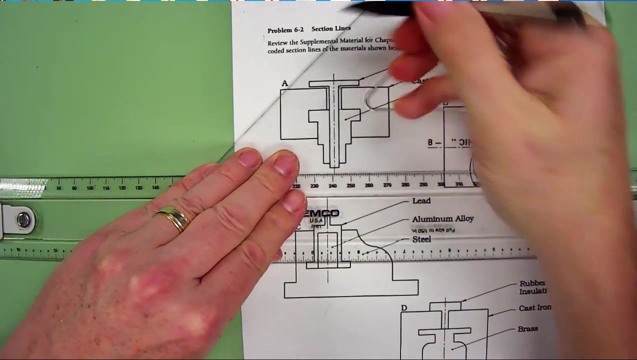 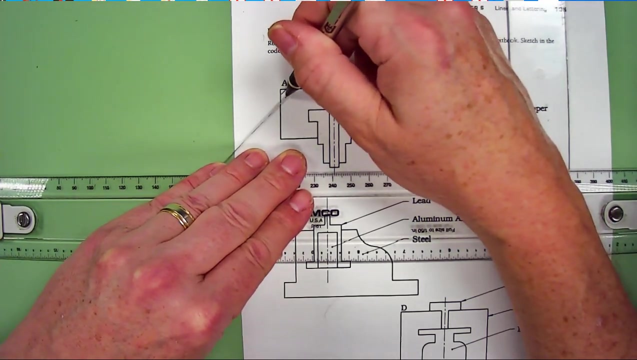 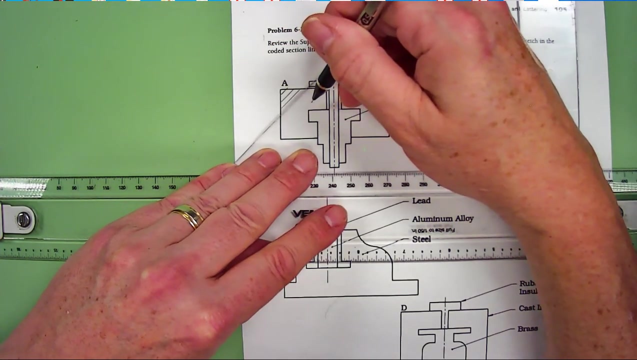 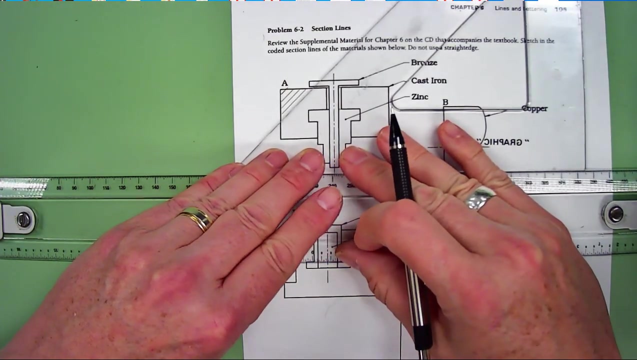 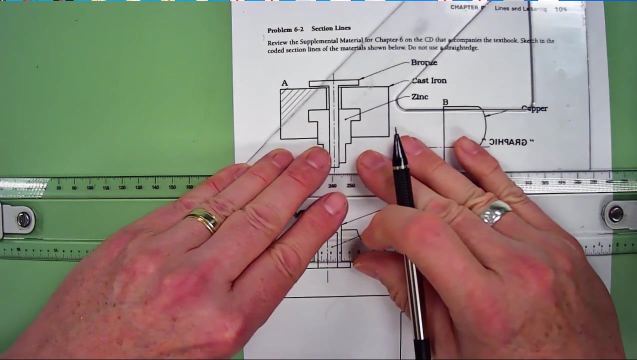 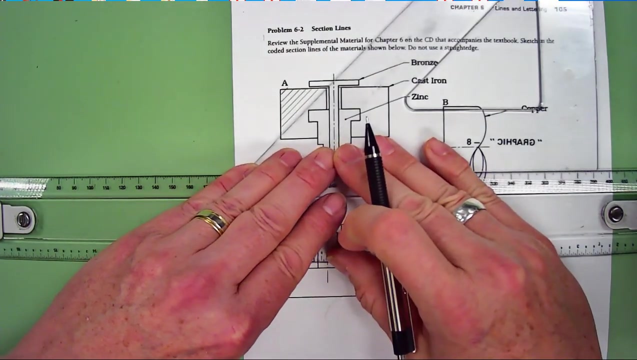 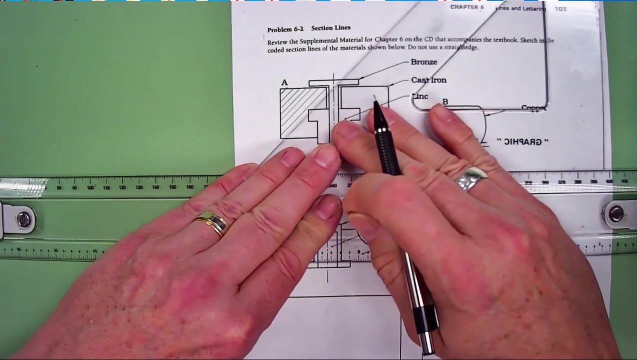 Let's see. okay, that's close enough for government work. now our cast iron lines are at a 45 degree angle, so I'm going to make lines. my head is usually closer to the hatching, but then I'd be hitting the camera and this is how hatching. 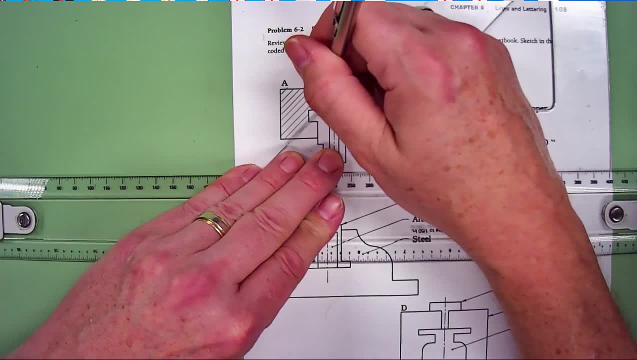 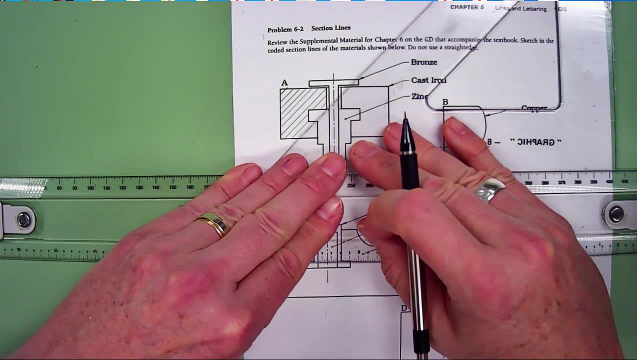 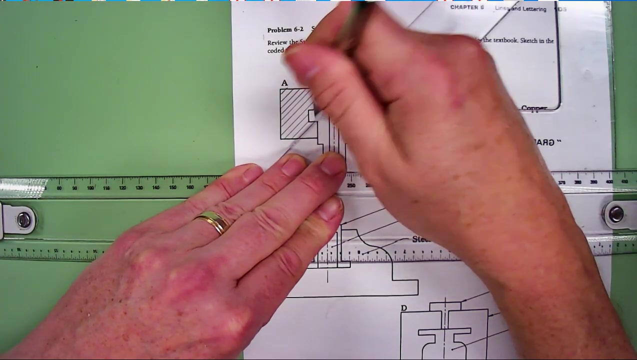 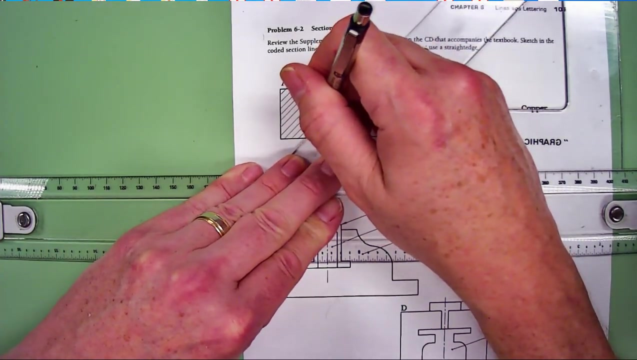 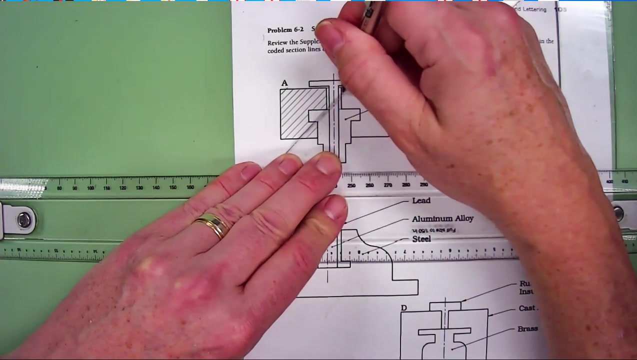 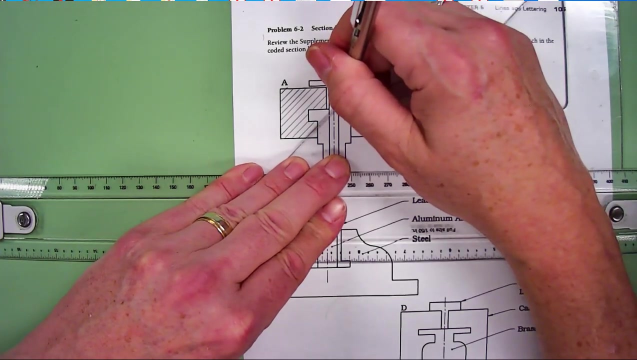 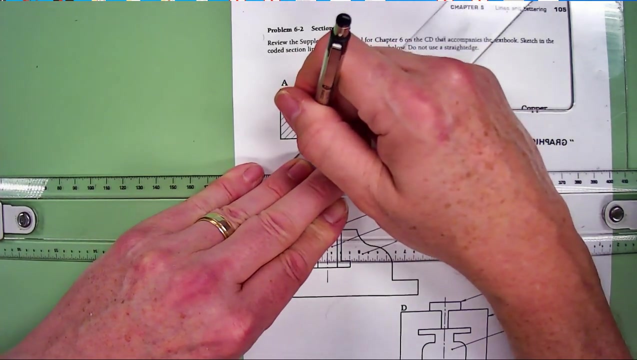 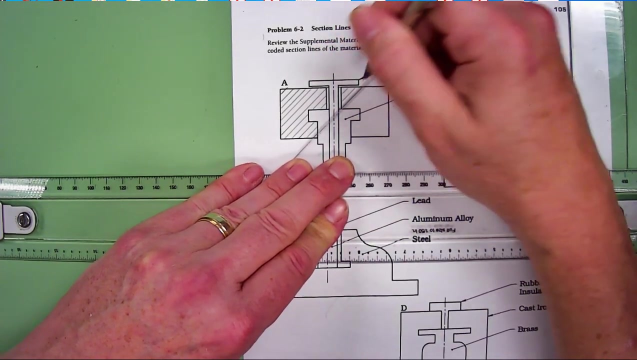 is done now. in a perfect world, I would have measured and made some starting lines. oops, I thought that would get away from me. see what I'm doing here. I'll go right over here because this is where it has to go, right here. you can sit here a little longer without finding a spot. oh, oh and then. 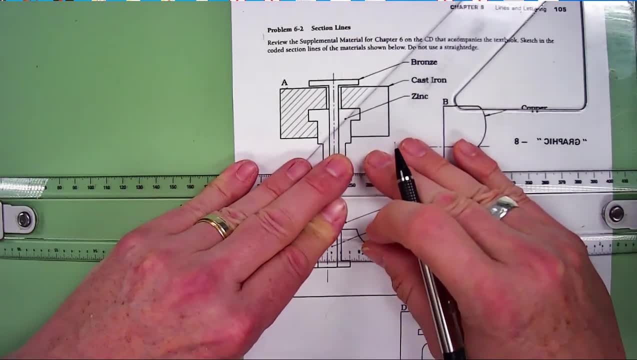 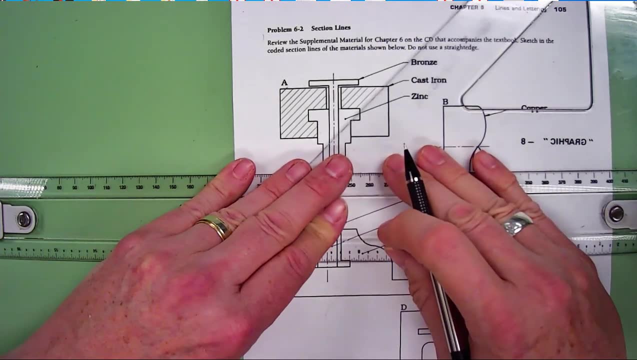 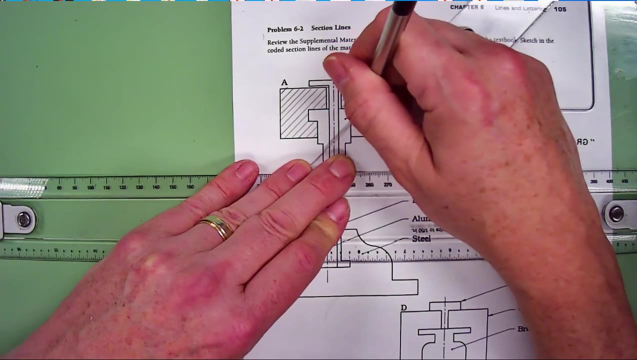 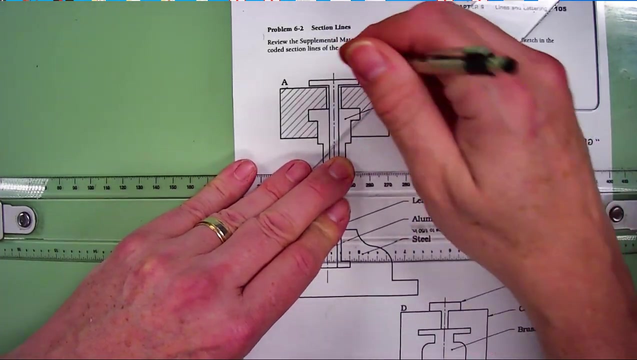 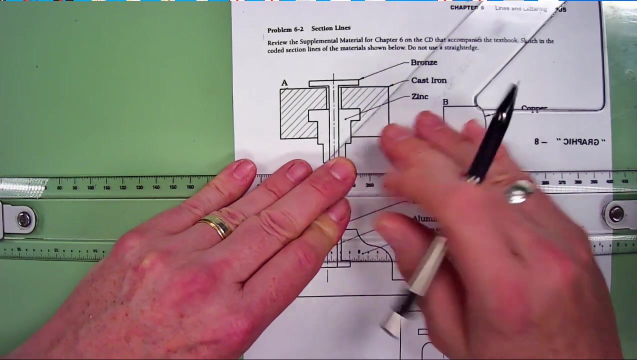 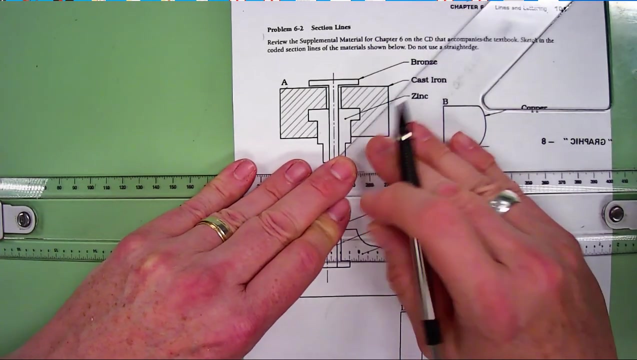 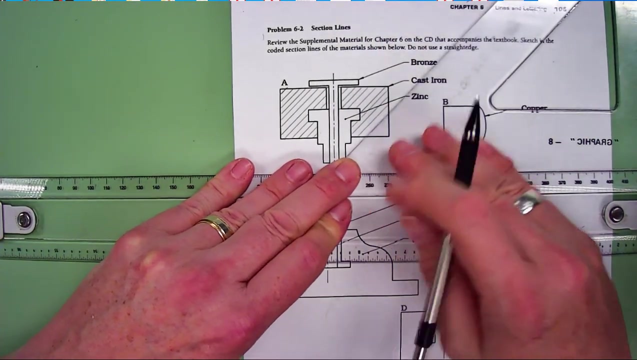 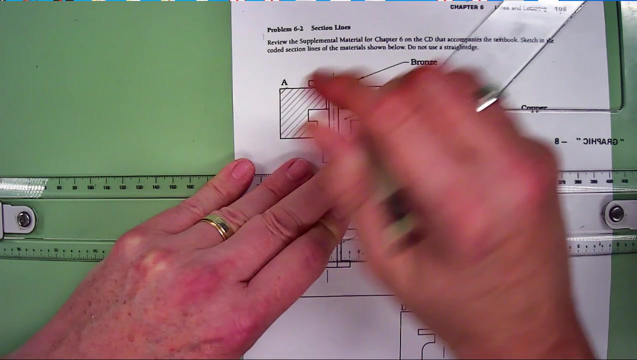 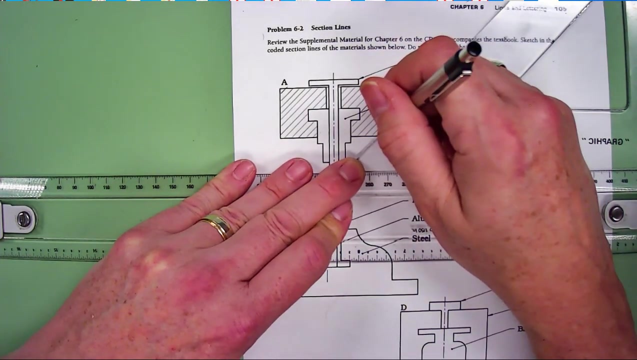 good, here I'm going to start hitting the books that I've got this on. But this is the proper use of your triangles. Patching should not be done free-handed. Use your straightedge as you can. I think I'm going to get this one completed. 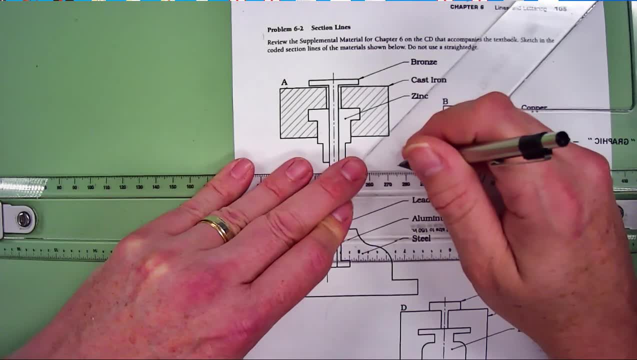 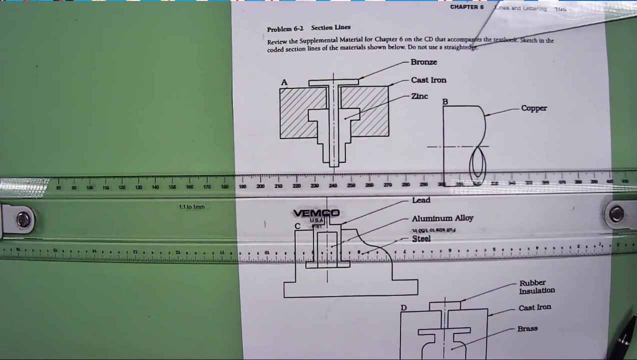 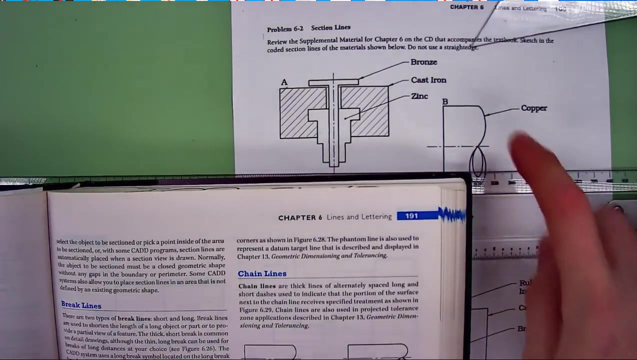 Okay, Yeah, Hot diggity dog. Okay, Now see how that looks. It's somewhat uniform. Again, I should have measured the distances and put tick lines where I should have gone. I'm going to cover this one real quick, because it's copper. 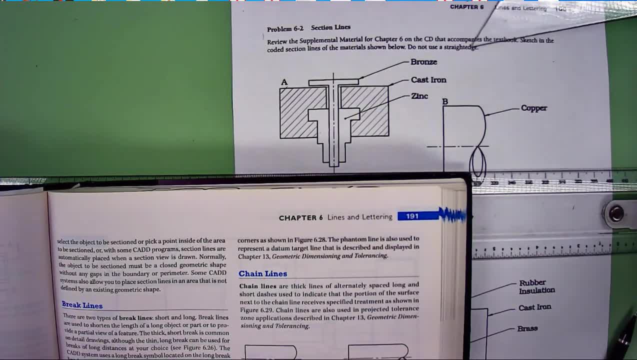 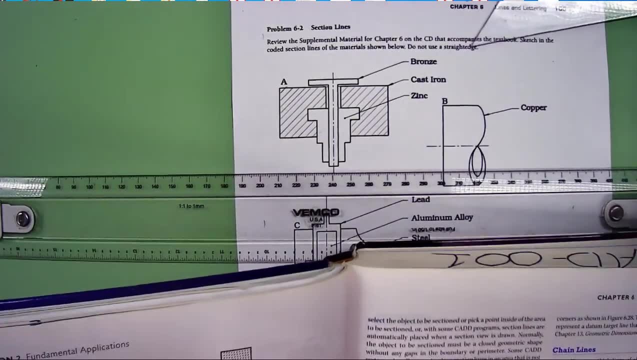 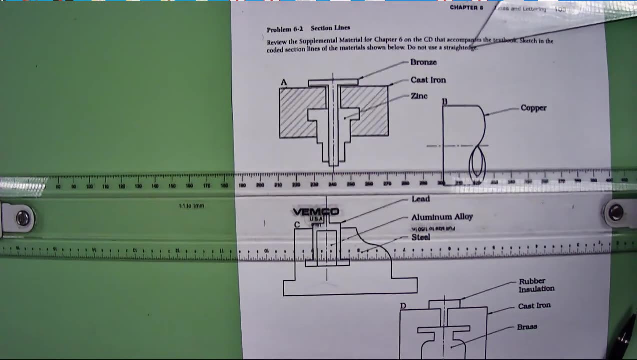 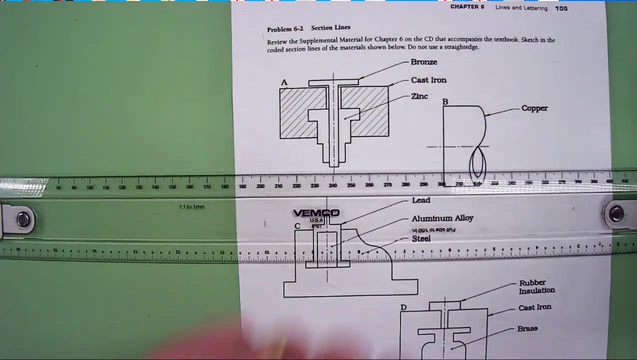 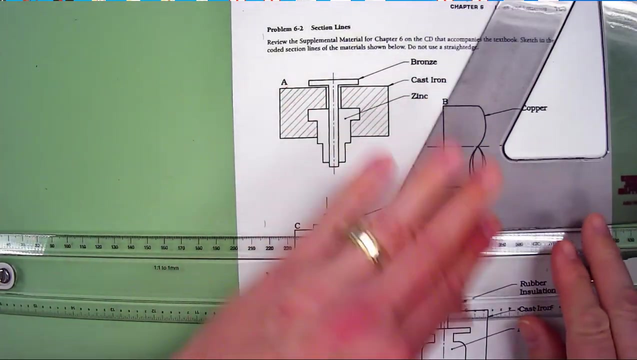 And I'm going to go ahead and do that. Okay, So that one is a line and then a dash line, and then a line and a dash line. So for this I'm going to use this one. I'm going to bring this down here. 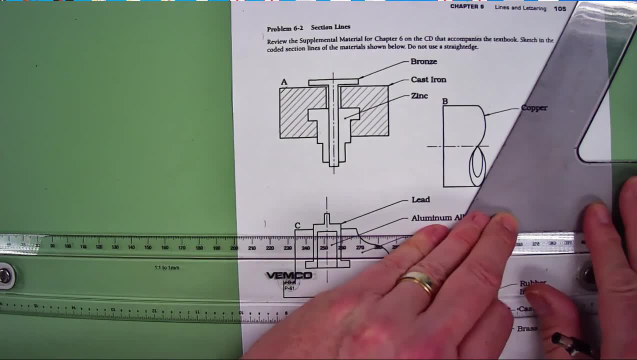 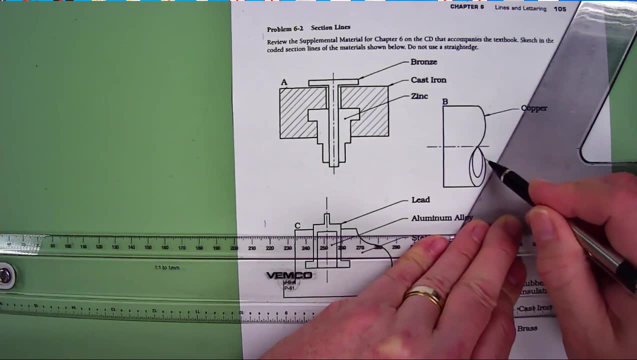 This one is different because the only part that gets hatched on this is this C shape, Because that's the only area that's cut. This is a tube. Okay, This is a copper tube, And it's telling you that because there is a center line through that. 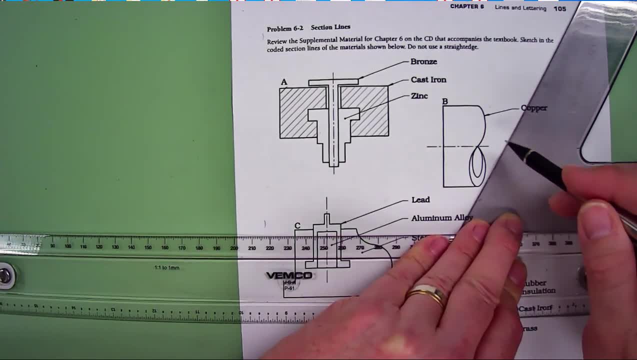 You only use center lines when you have a tube or a hole. Okay, And since this is showing the figure eight, Okay, Just trust me, There's a section over here that looks like an eight, But this would be the part that gets hatched. 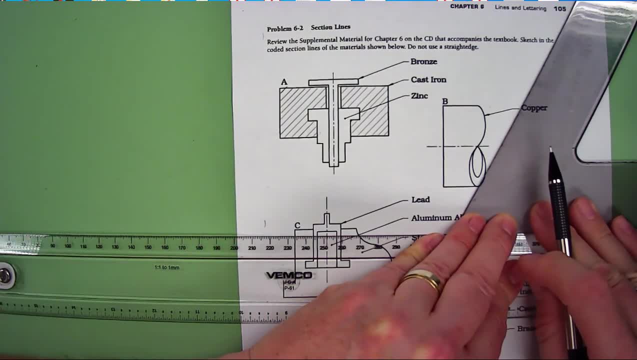 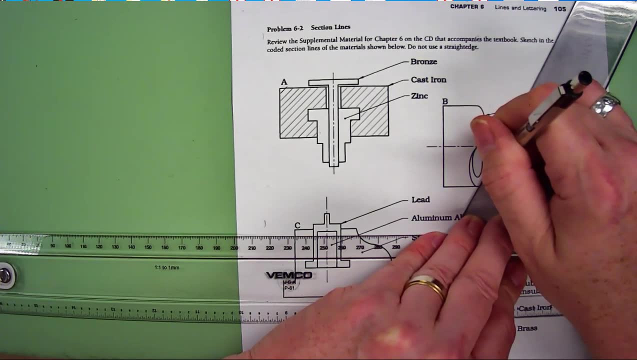 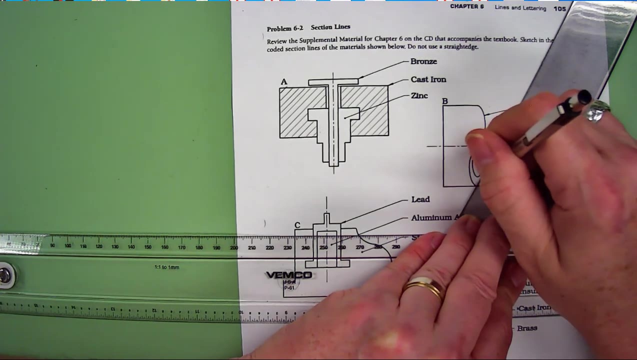 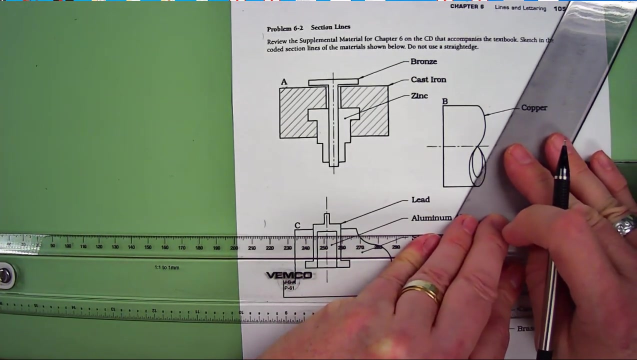 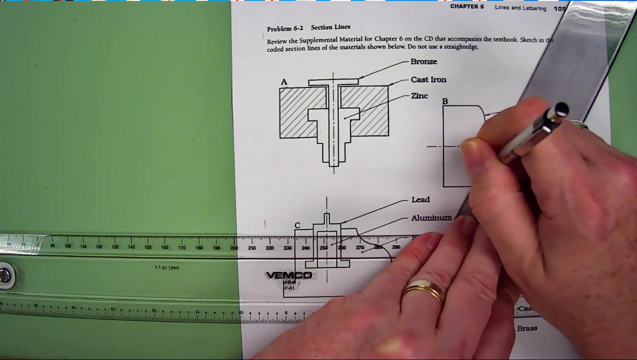 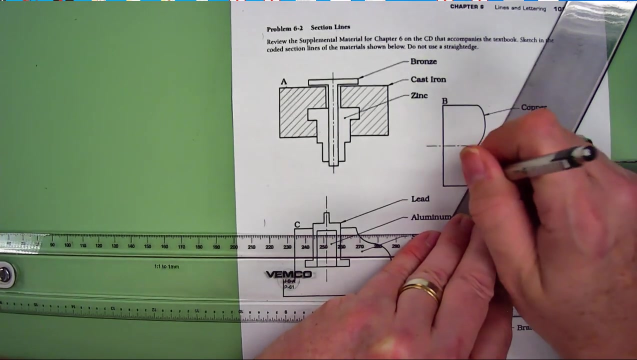 So we are going to: Okay, There's that, And then we go: Now, let me see, That needs to be right about there. So then we're going to go here And here. Okay, See that, And then we're going to go. 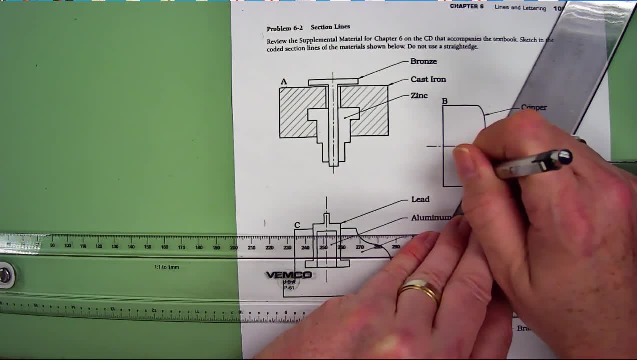 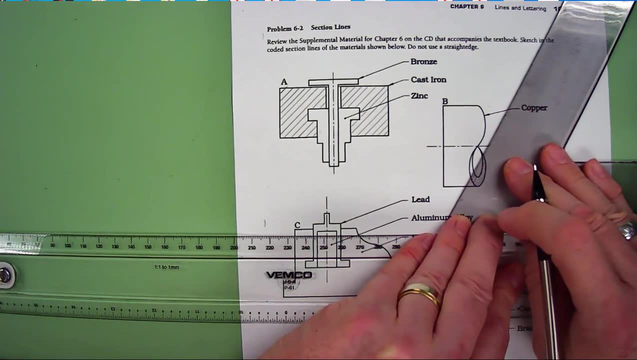 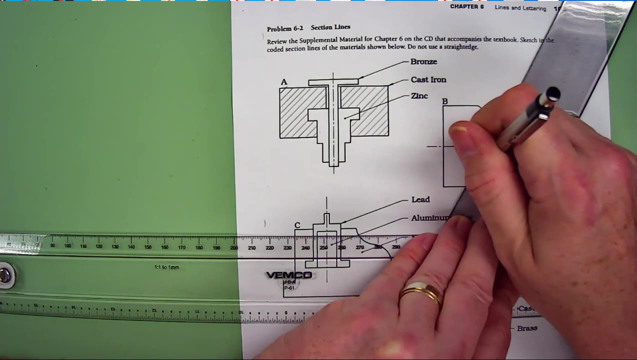 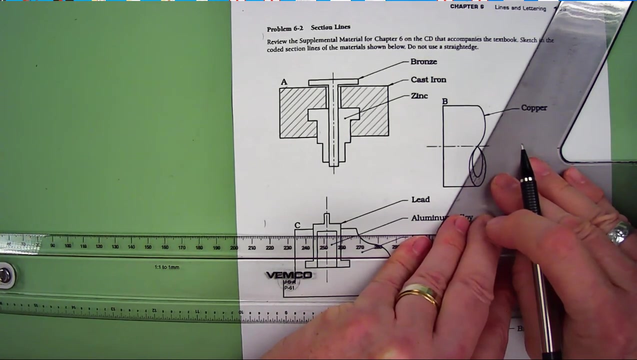 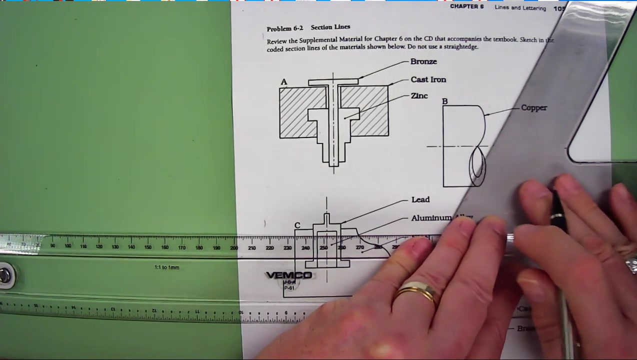 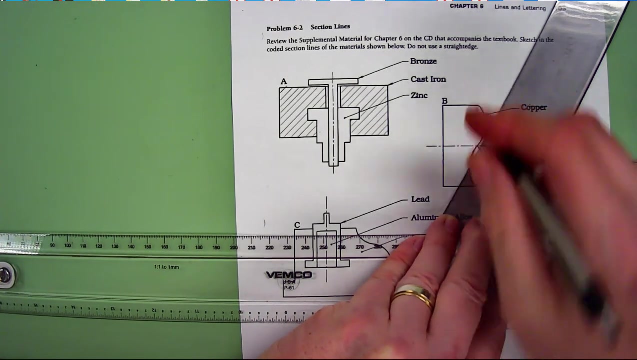 Make some very small dashes And then Solid line. Now I don't have anything left to draw on that part. So now we're going to have some very small dashes, Can you see that? And then one more line should do it. 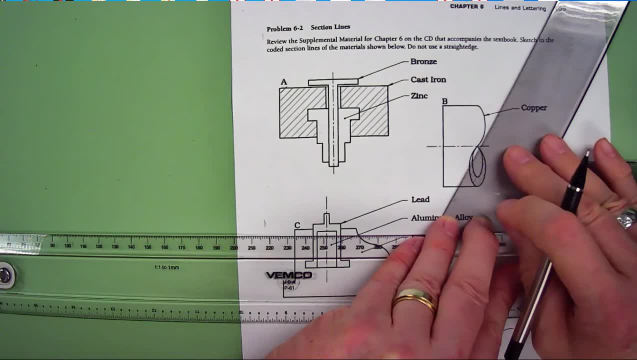 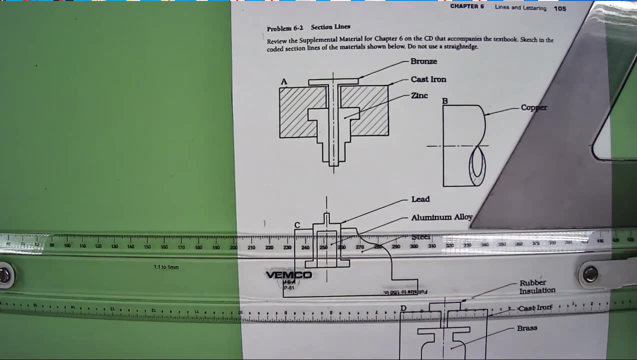 Because when I move it up here we don't have anything left. So that will be all that. you hatch on that one, Okay. So now that that's out of the way, I want to get back to the bronze Bronze is the same as the copper. 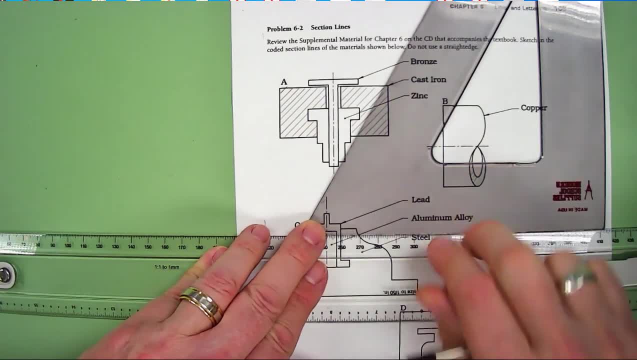 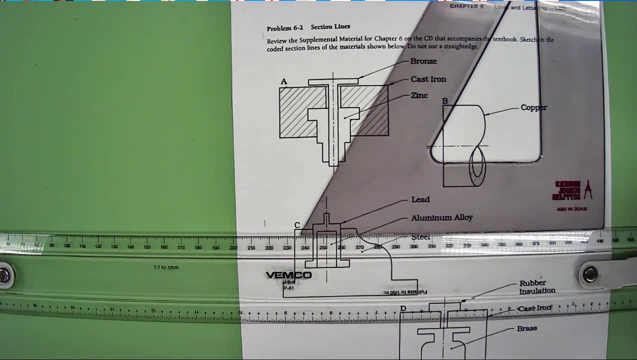 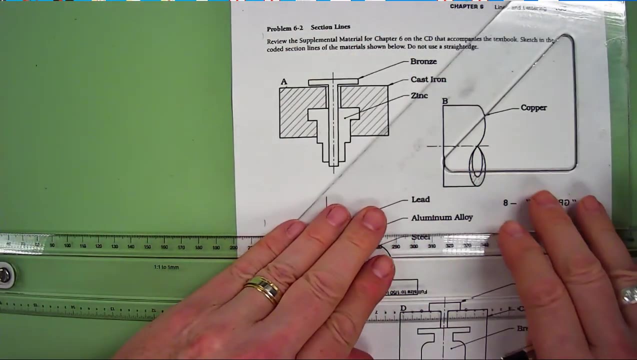 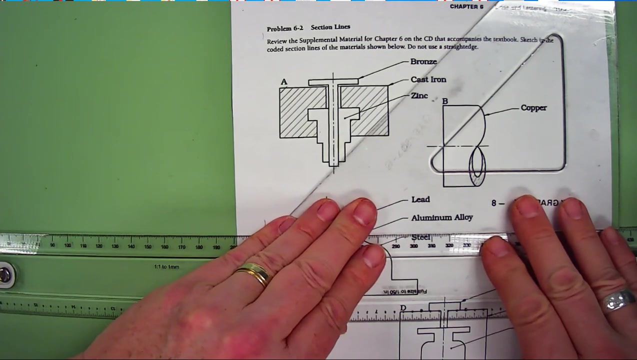 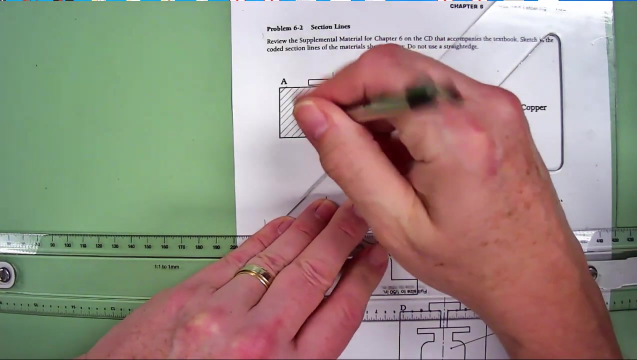 So that's going to be fairly easy right here Now. Okay, Now I'm going to go back to my 45 instead of using my 60.. Okay, And Let's see From bronze. I'm going to start right here. 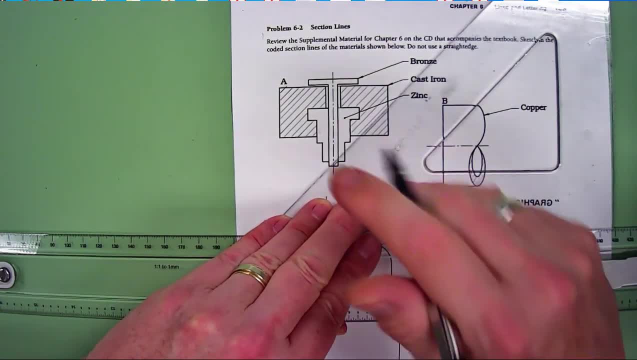 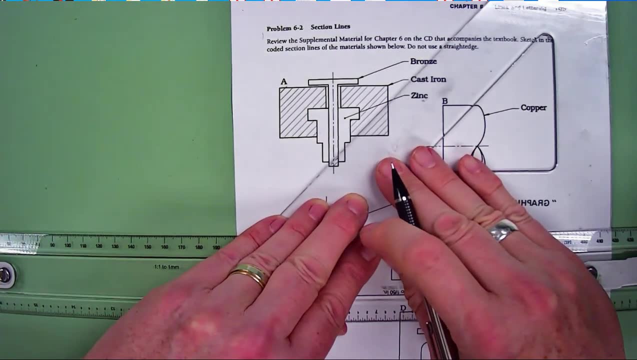 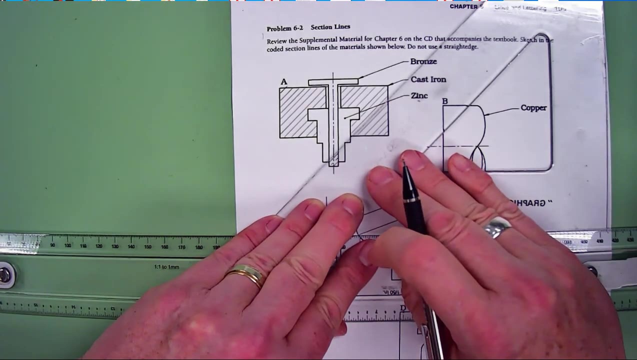 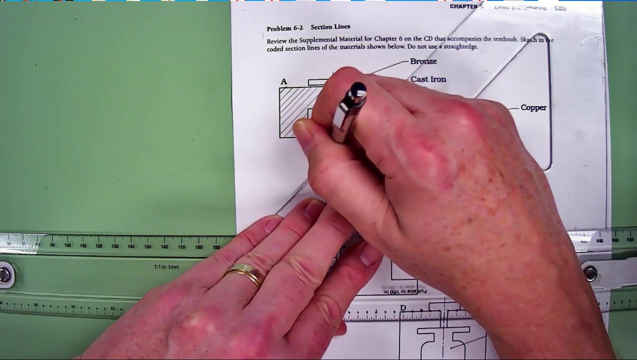 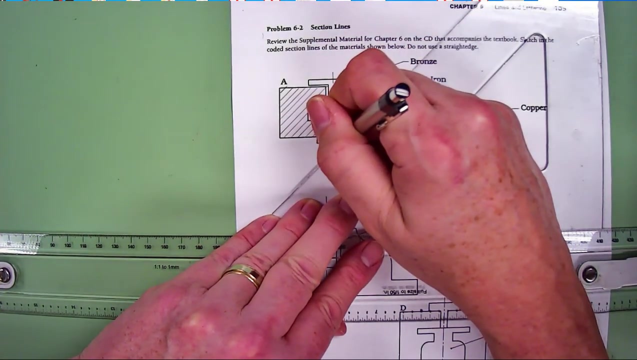 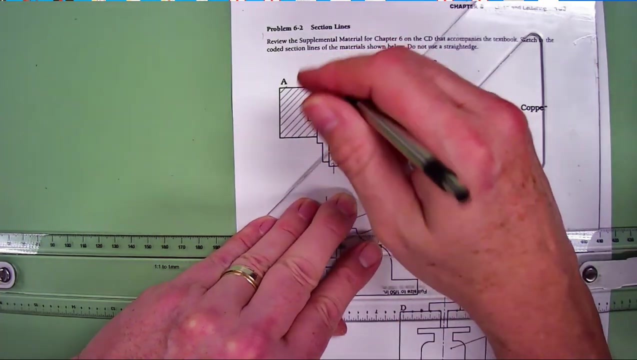 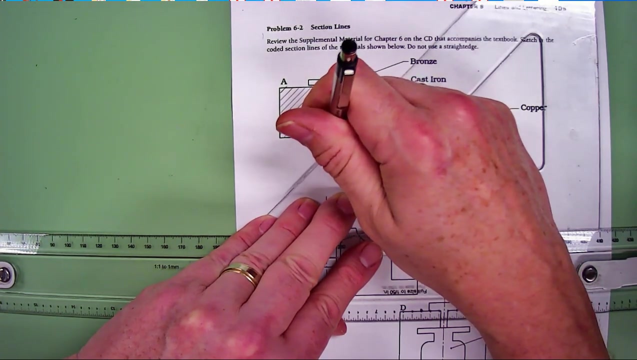 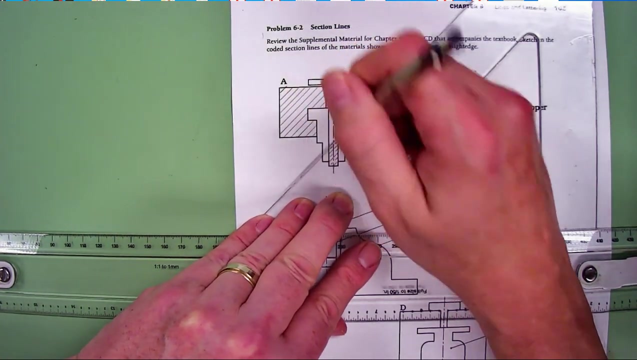 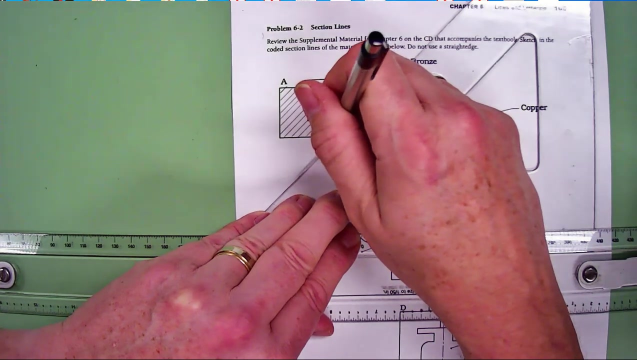 Okay, Correct, And Of course. So that's very well, einen Kyle, But we have to keep that clean. So, Ah, There it goes Once. Okay, Hatching and lettering are going to be the most time consuming, but typically the 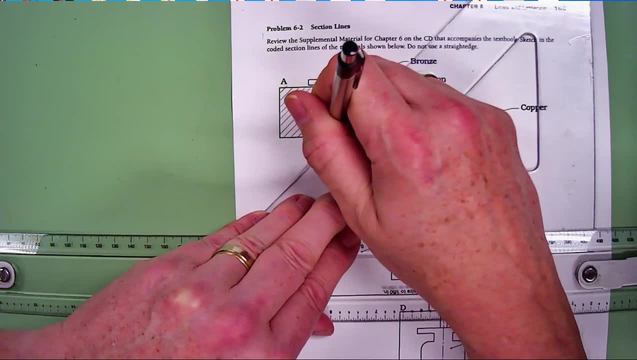 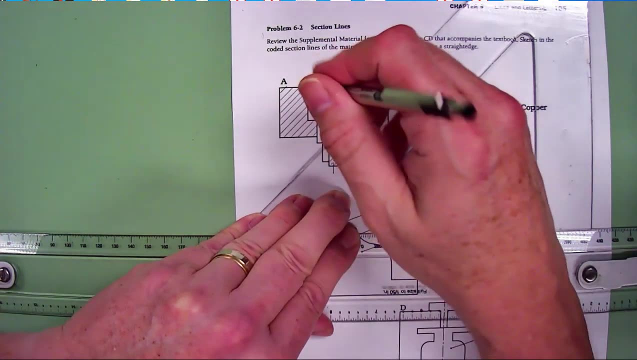 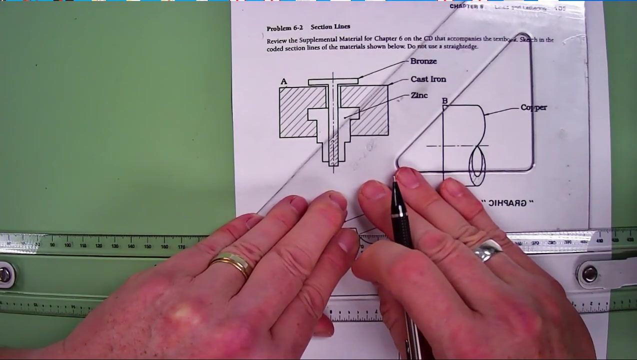 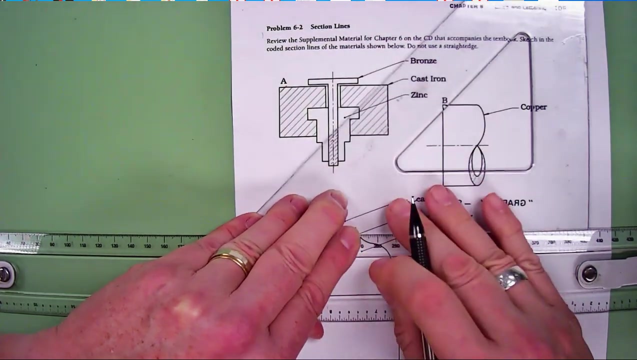 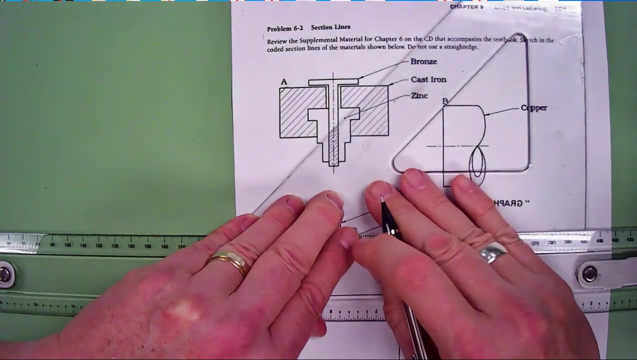 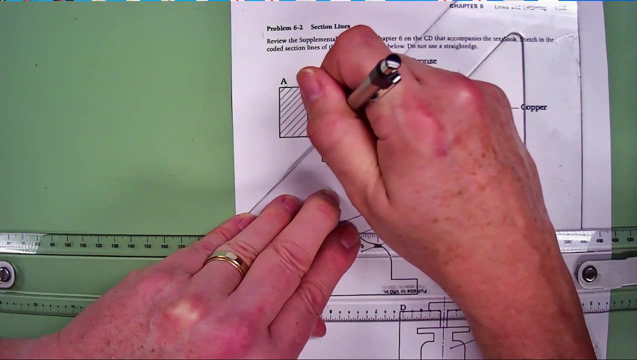 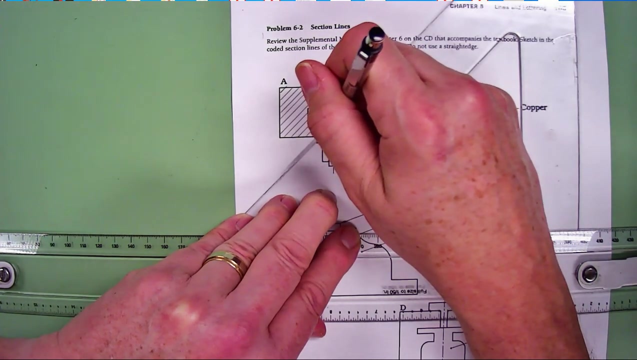 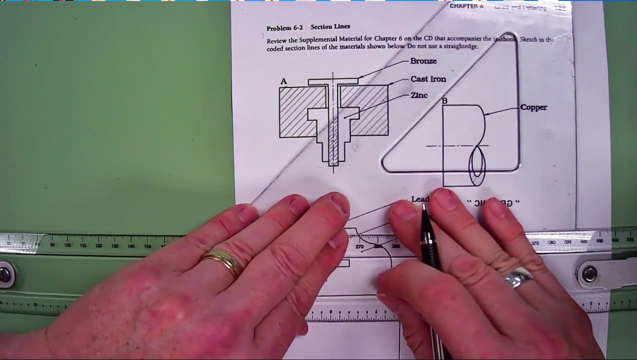 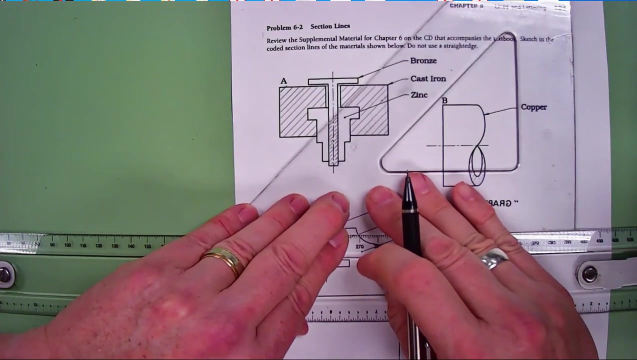 most rewarding part of board drafting, because if you do it right and do it with precision, it's going to look outstanding. I'm not saying a whole lot, but I'm trying to concentrate on what I'm doing here. It has been a long day. 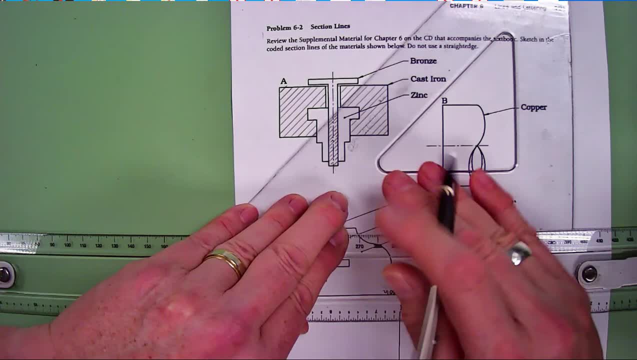 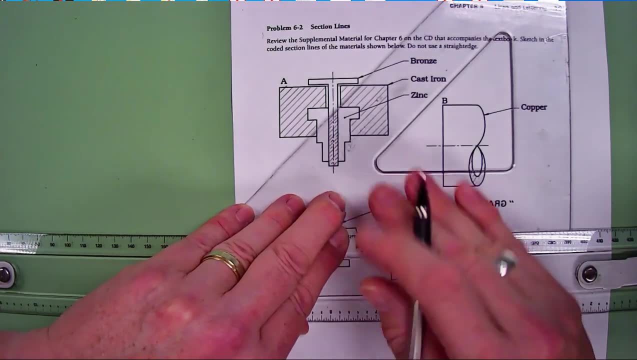 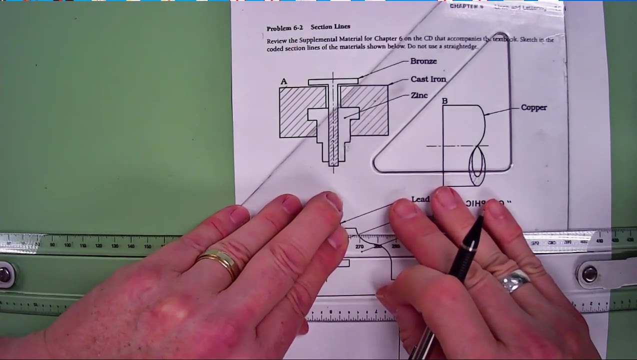 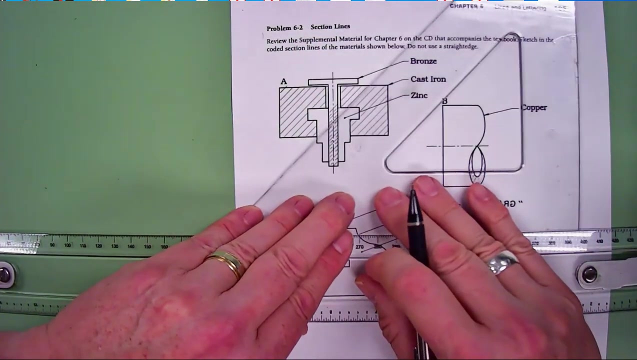 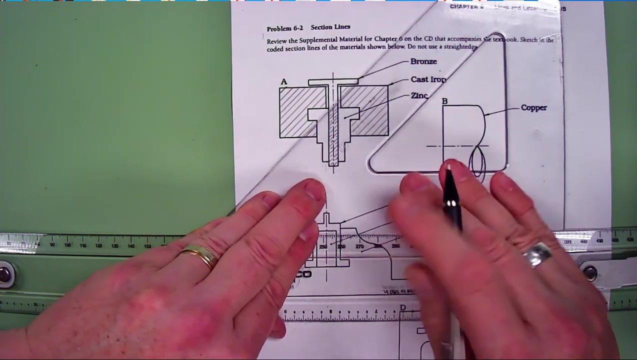 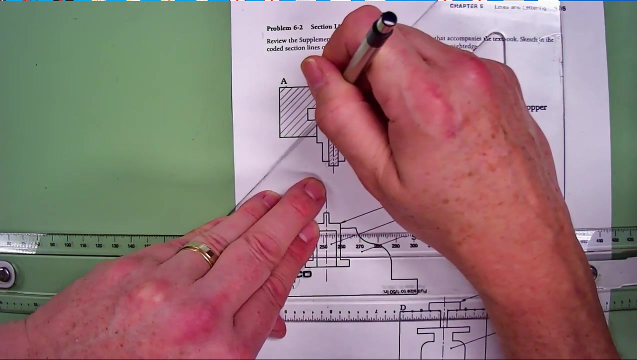 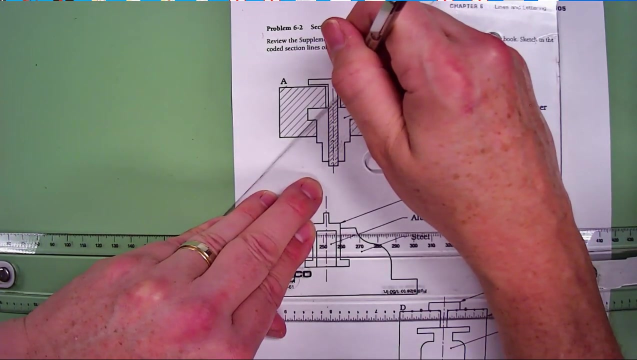 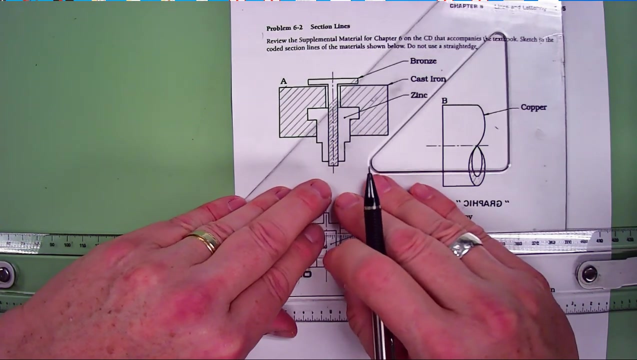 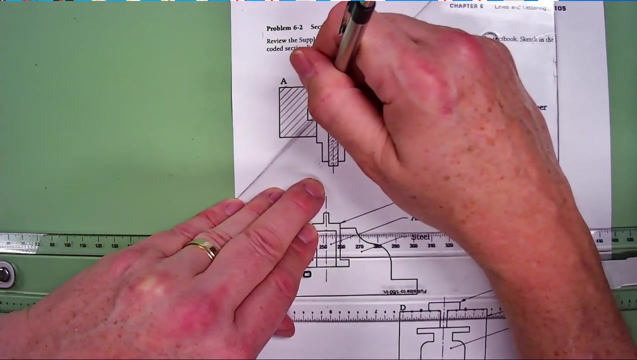 It's not a long day. It's been a long time since I have physically done this. See how it's looking. So then, when you start up there, you need to remember to: Okay, Okay, Do your dashes up there as well. 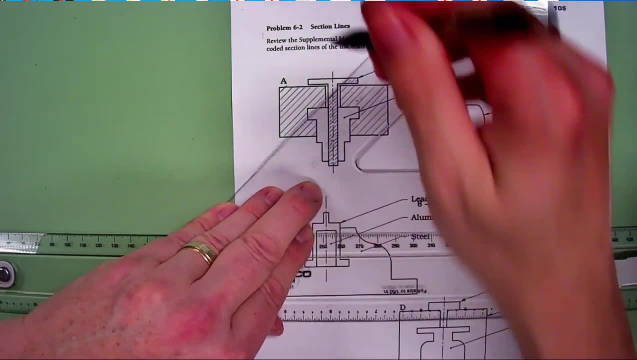 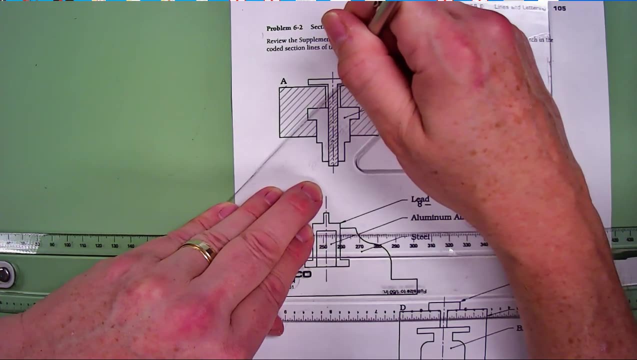 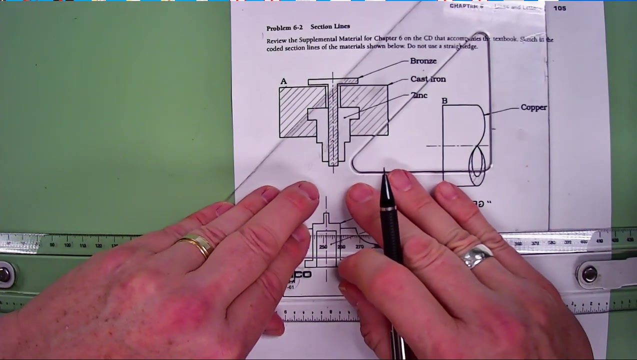 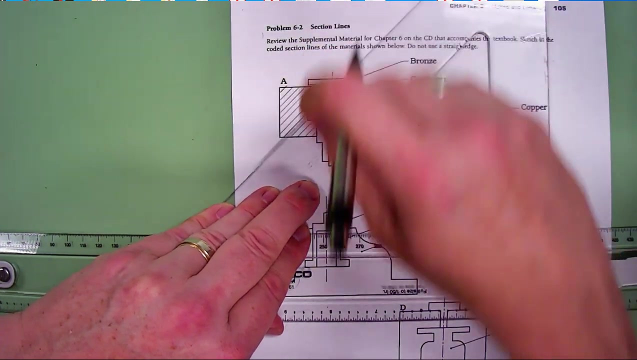 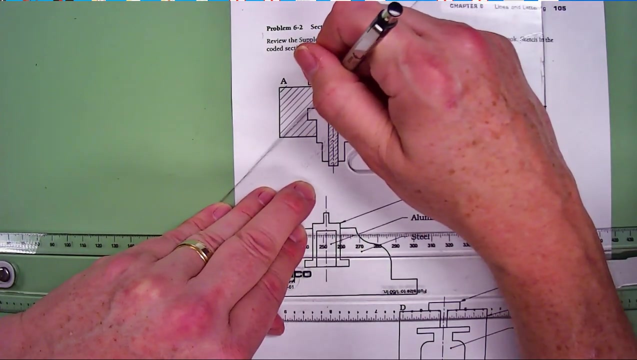 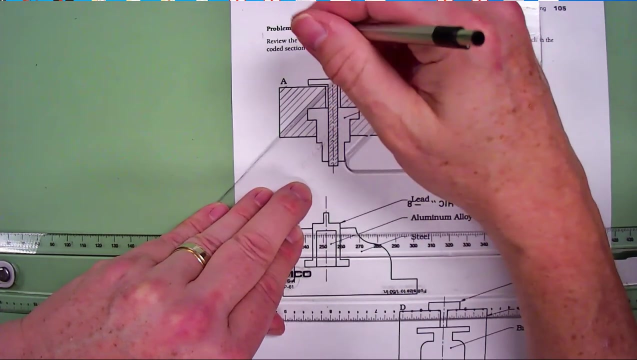 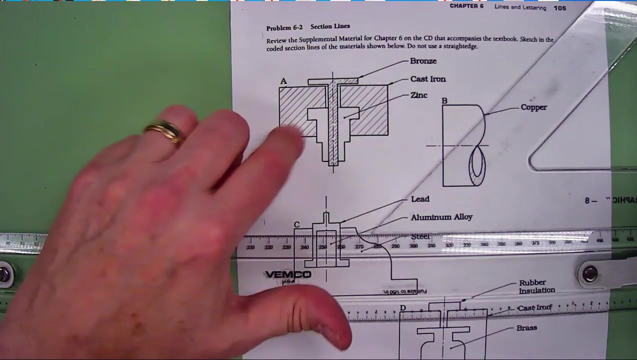 If you make a mistake, you can always use your eraser shield, And that'll keep you from messing up anything else you have. I'm going to stop at that point, right there, Because you get the idea. Okay, And then for zinc. 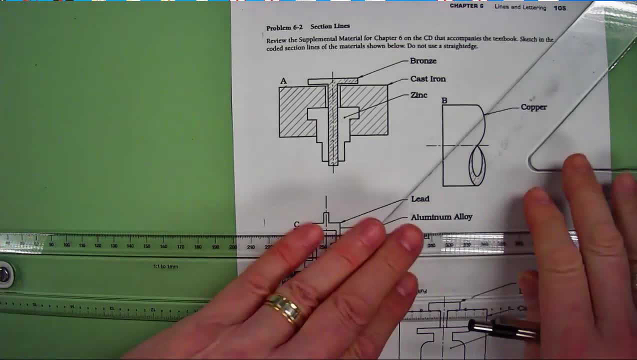 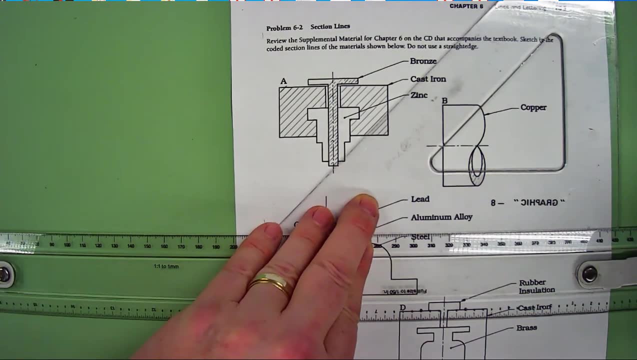 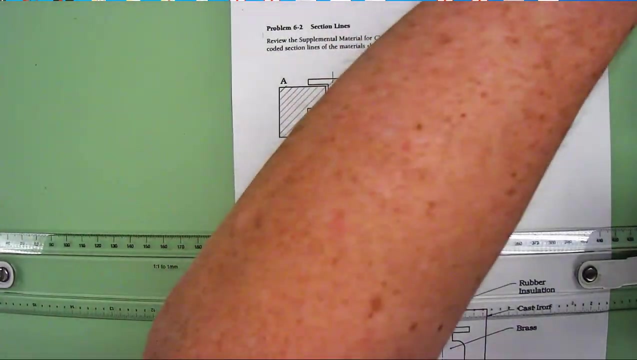 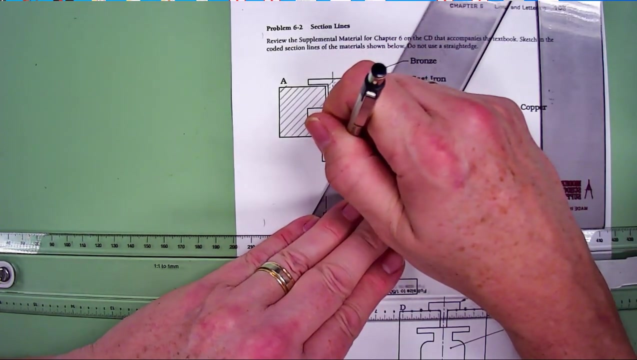 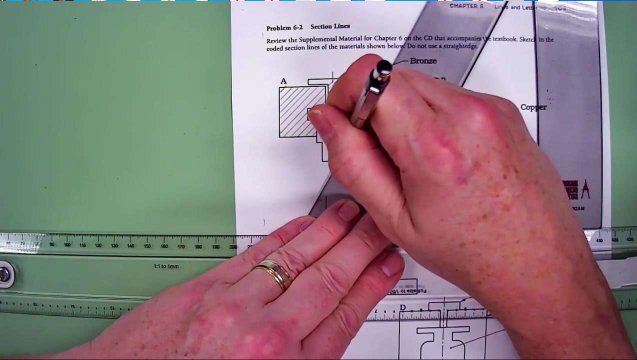 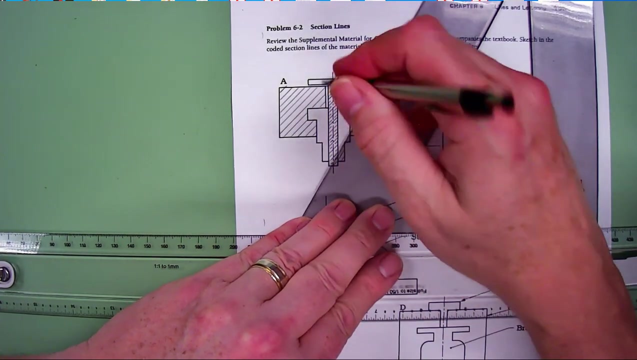 Zinc is a crisscross. So what we do, What we do, I'm going to- Since we've got so many hatches, I'm going to draw one on top of this one, of this one And use it, Okay. 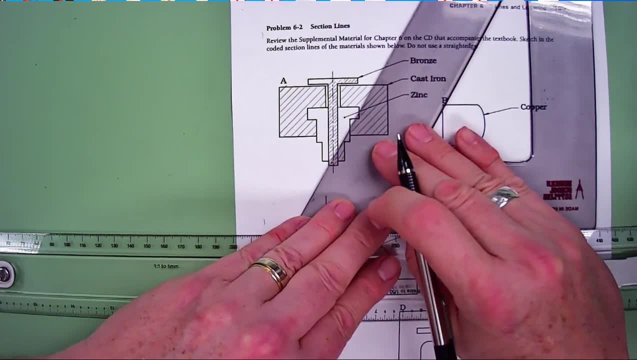 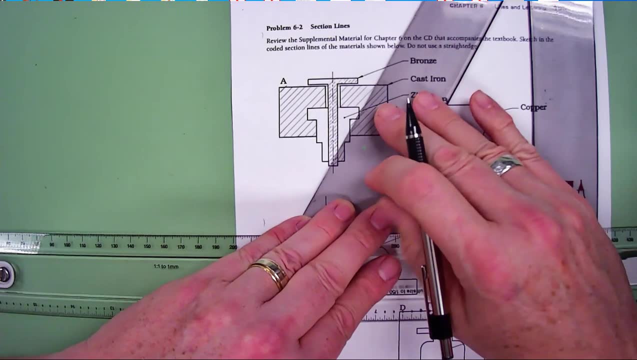 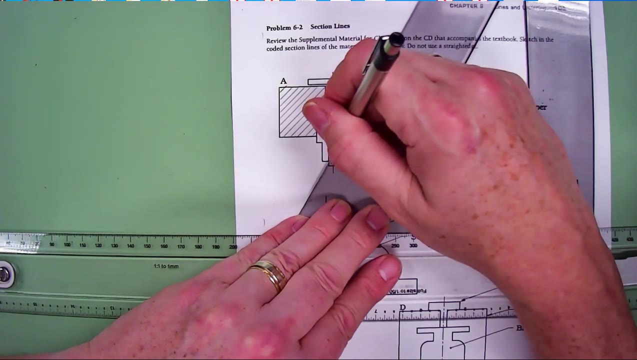 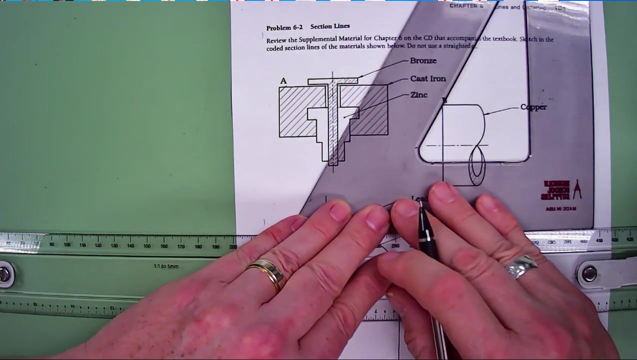 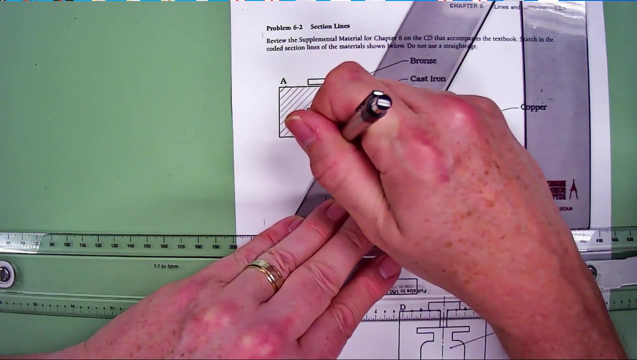 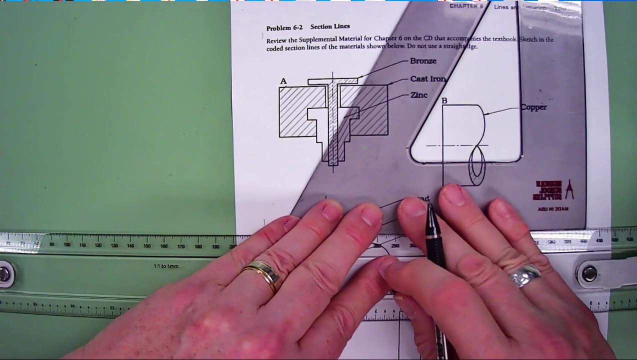 All right, Let's go. Let's go, Okay, Okay, Okay Okay, Because you don't want your hatching to be confusing with the other lines And I'm only going to do to the top of the right side of this. 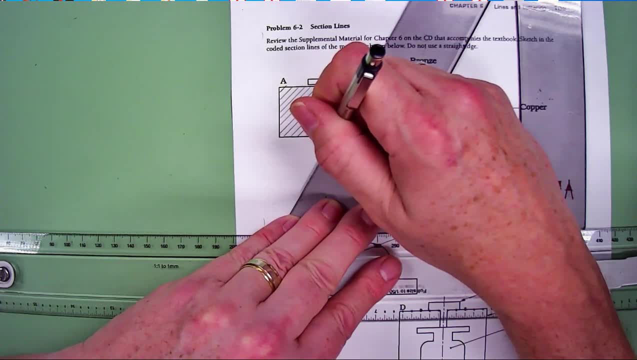 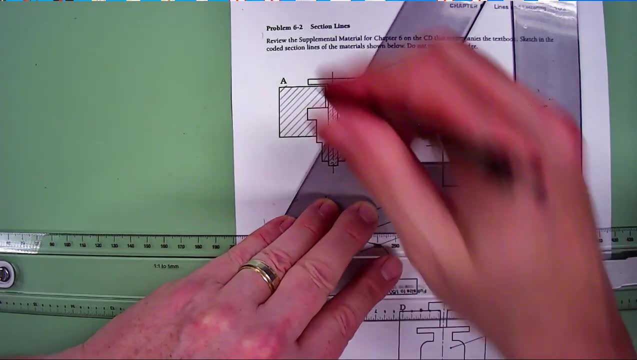 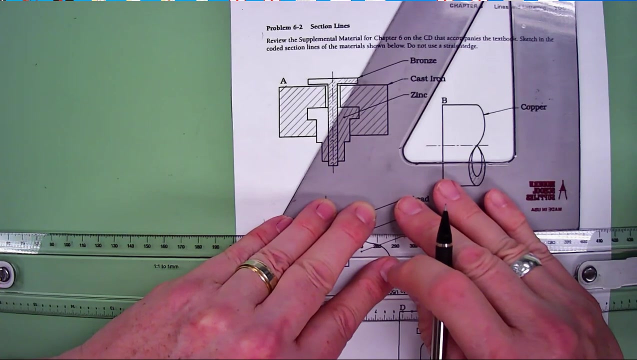 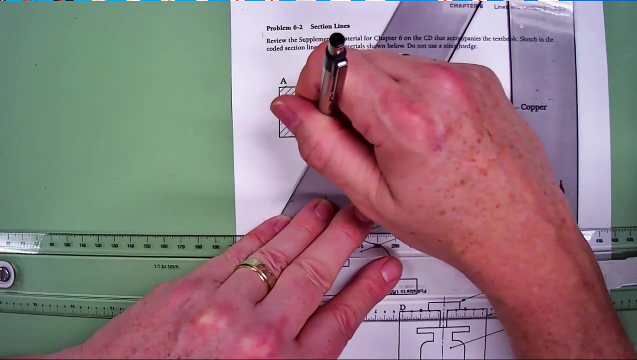 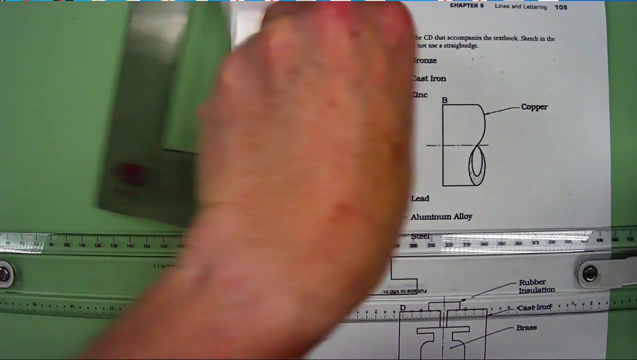 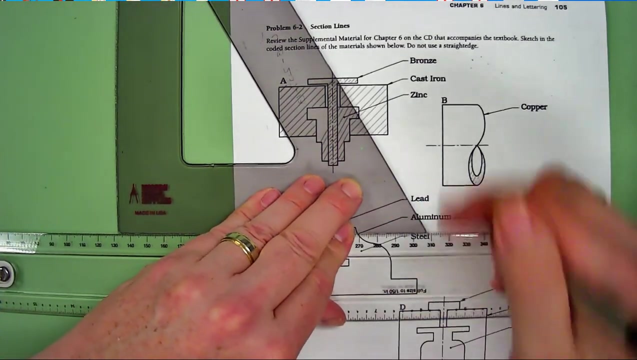 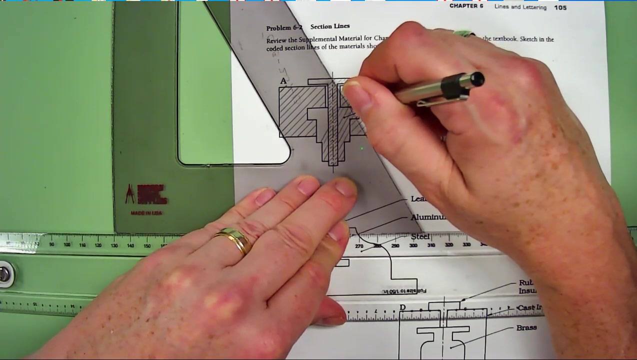 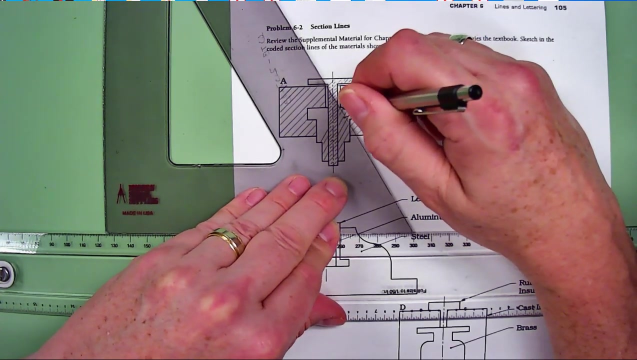 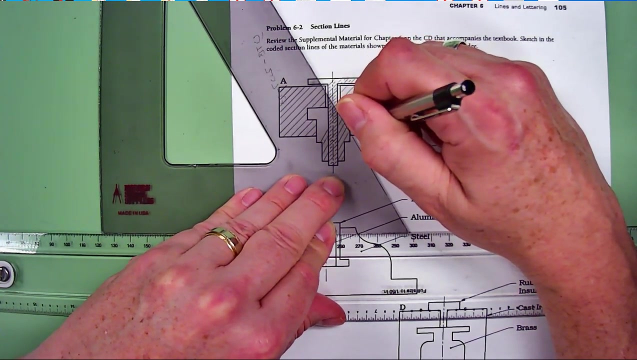 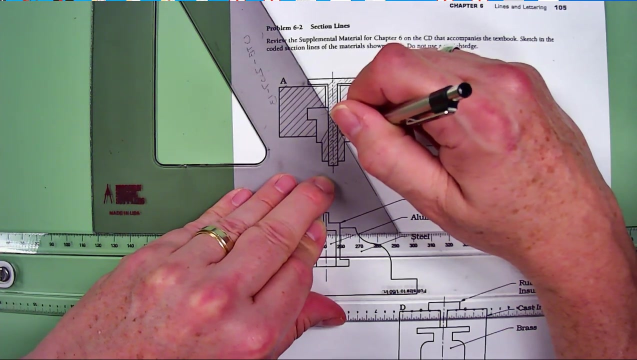 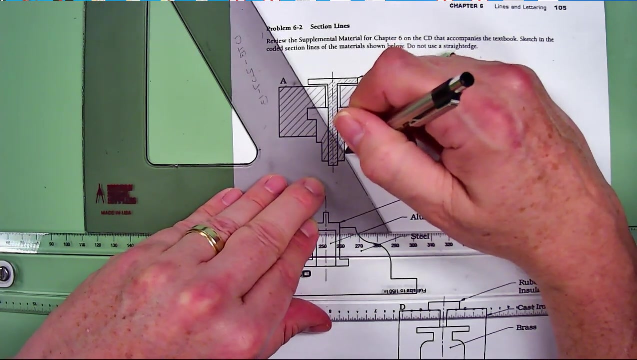 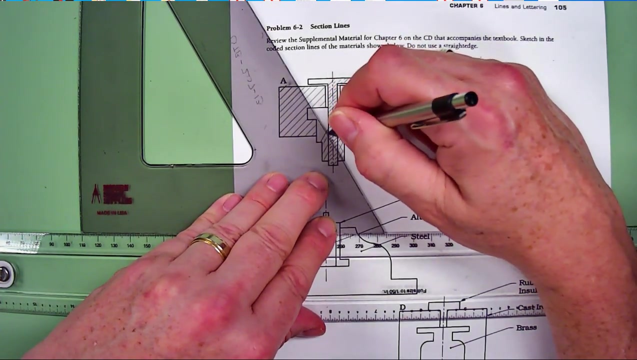 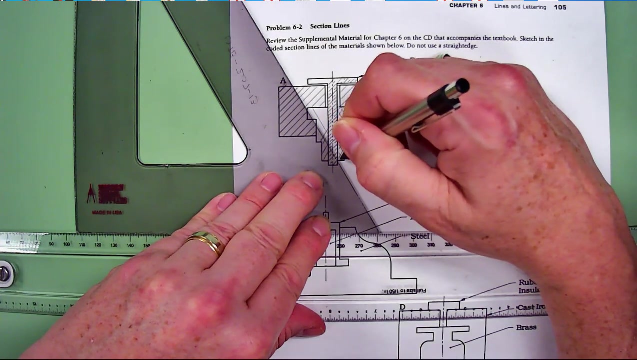 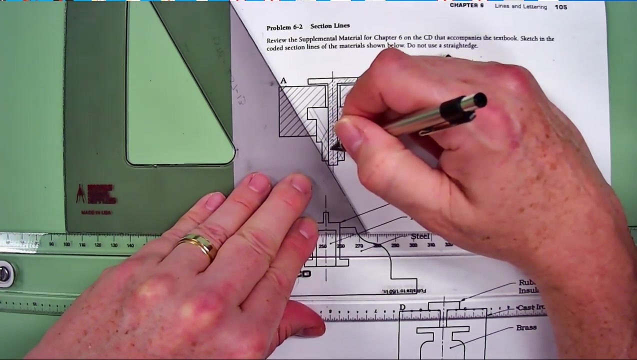 And I hope that's okay, Because then that's when I flip my triangle and do the rest of the crisscross. So we just grab this guy And go back to this, And go back to this And you see how those are. 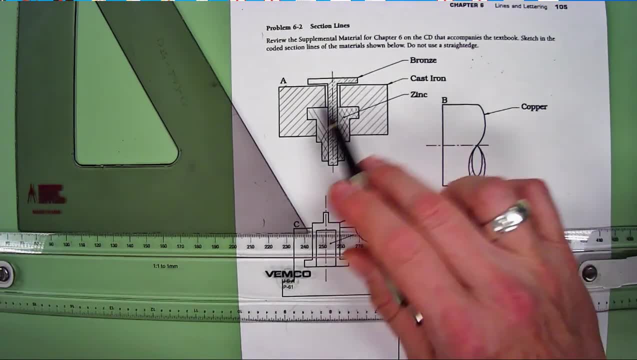 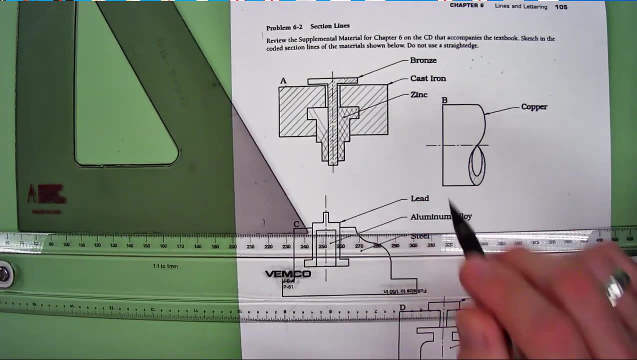 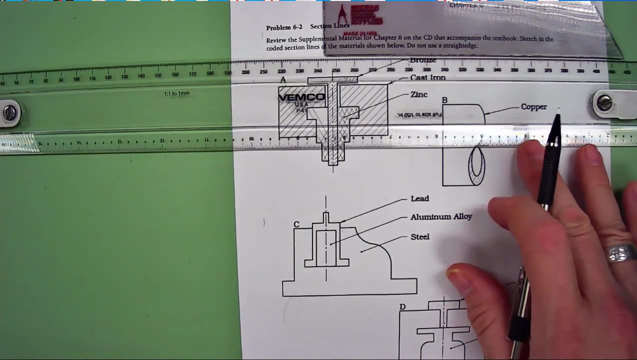 So that's how you differentiate the different metals in a drawing: Cast iron- And, like I said, I should have measured those. And it's easy to do that if you will set up a series of marks, And they don't have to be dark. 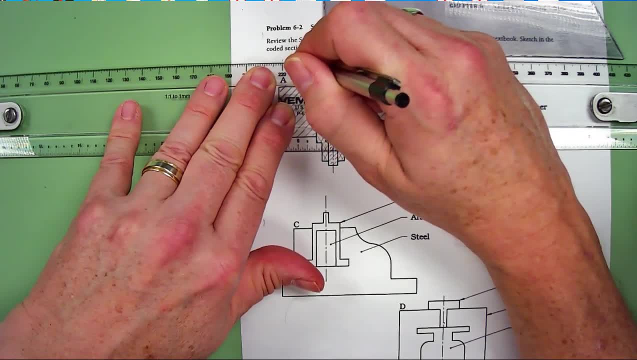 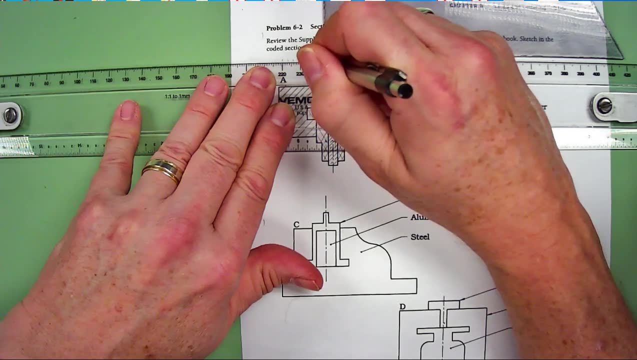 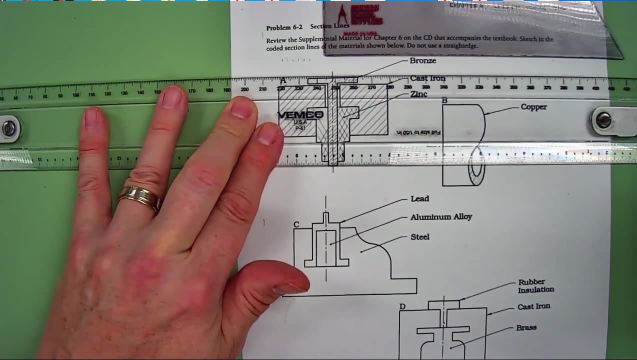 But if you want to set them up every, say three, Every three millimeters, See, That would cover. See the little lines I made. Can you see those? Because the idea is to make them faint And then erase them when you're done. 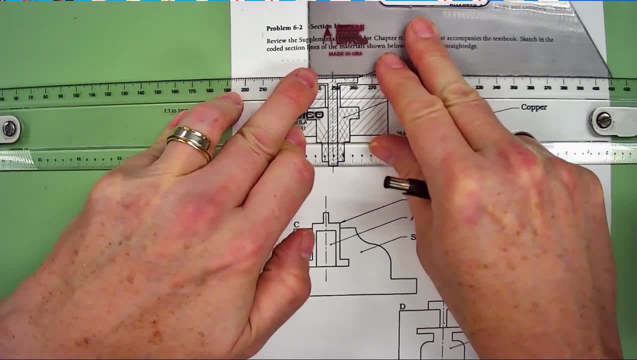 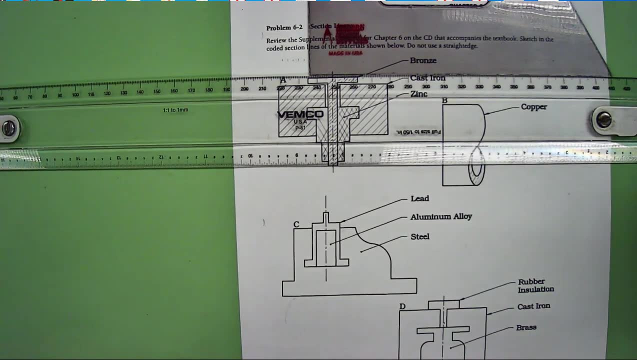 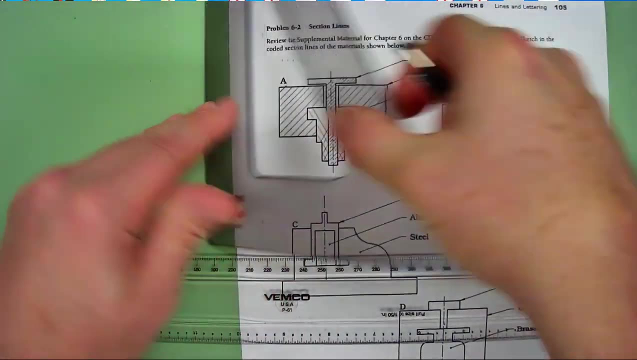 Excuse me, And then you can use that to line up your triangle. Okay, For wherever you're going to be putting them. Okay, Putting the lines And that line. Those lines can be used anywhere on your triangle. See Like I can put in a line here. 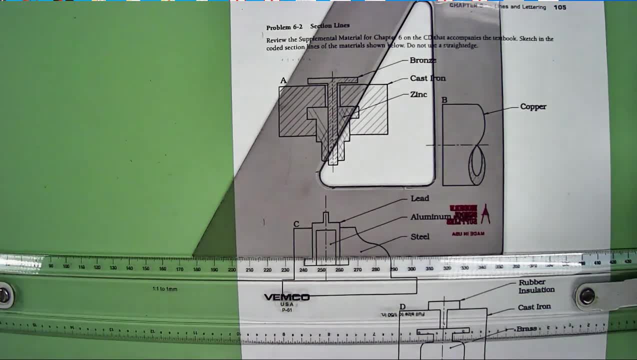 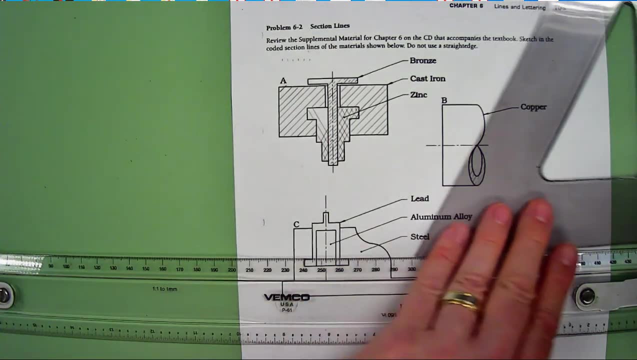 And in a line here And in a line here, And that would keep things all nice and even Kind of like how I was doing with the copper or the bronze Okay And the copper Okay. So I hope that helps you out. 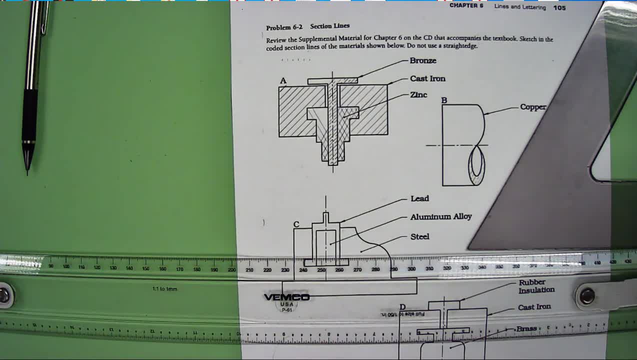 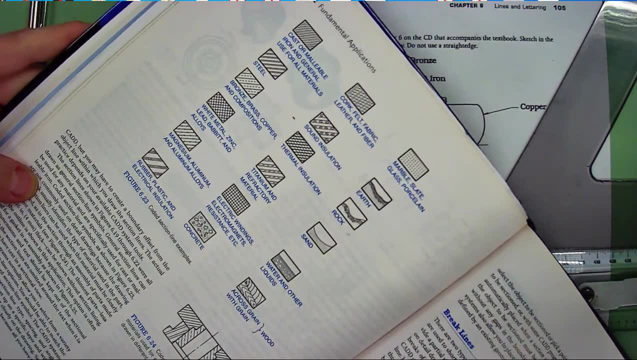 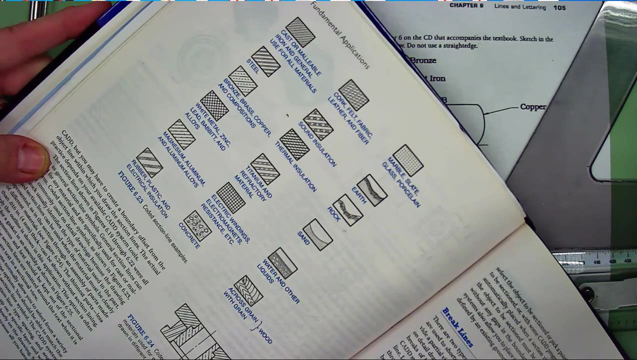 I don't want to do all of it. I mean it's fairly straightforward. But, like I said on page 190 in the textbook, Okay, There are all of your various metals and how they should look, And you know you can use that as a reference guide. 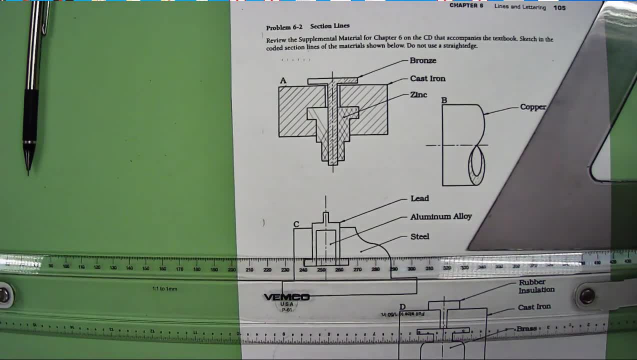 Okay, So let me know if you have any questions, And again in this book, just in case I get some people that are not in my class But still want to know about how to have them, I'll be happy to answer. 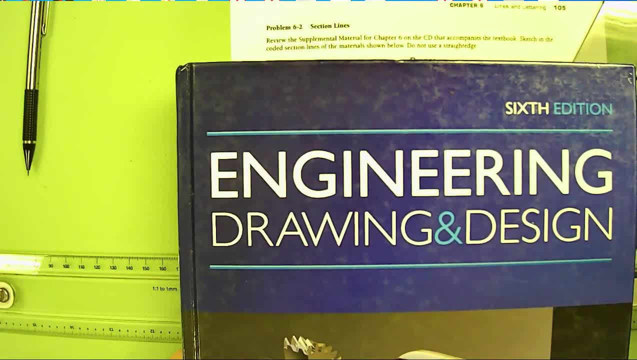 So, as I was saying, if you have any questions, Let me know, I'll be happy to answer And I'll see you guys next time. Thank you, Bye-bye, Bye-bye, Bye-bye, Bye-bye. 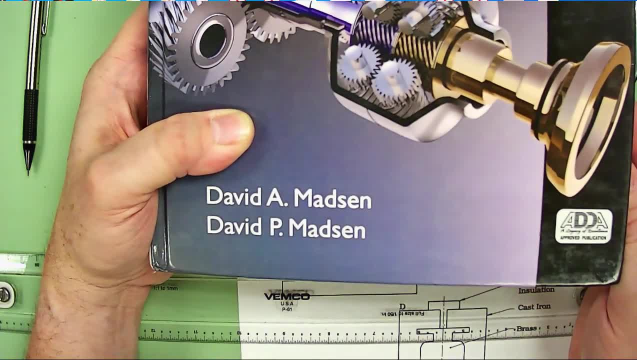 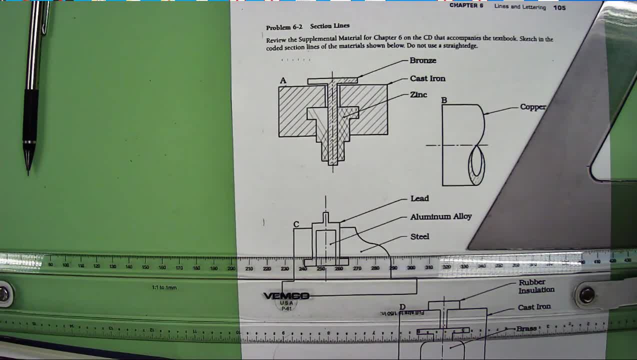 Let me know if it isn't. Okay, I need feedback, So help me out here. Thanks a bunch And, as always, holler if you have questions. Thank you,